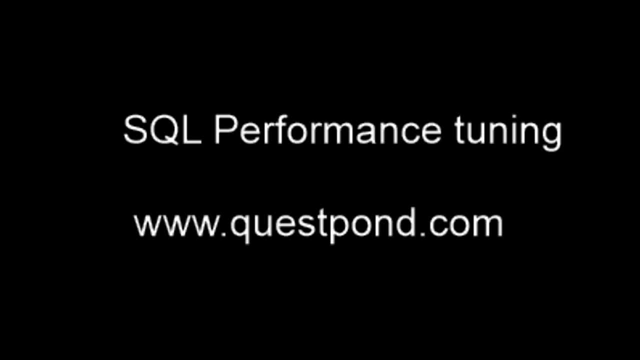 Good evening, Amar Abhijit Ravi Kim Harish. Today's topic is SQL Server Performance Tuning. This is going to be a one hour of session wherein I will try to stress on important points of how to go and fine tune SQL Server, what we should look at. Definitely a one hour. 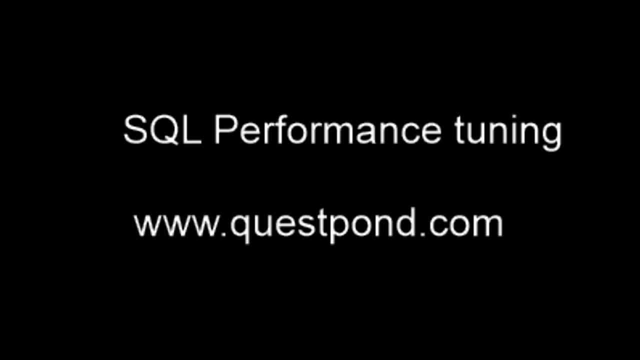 session is not enough for topics like SQL Performance Tuning, but let us try to do the best what we can in this one hour. Before I start, let me know if you can hear my voice. If you are able to hear my voice, please put on the chat. yes, sir, we can hear you so that. 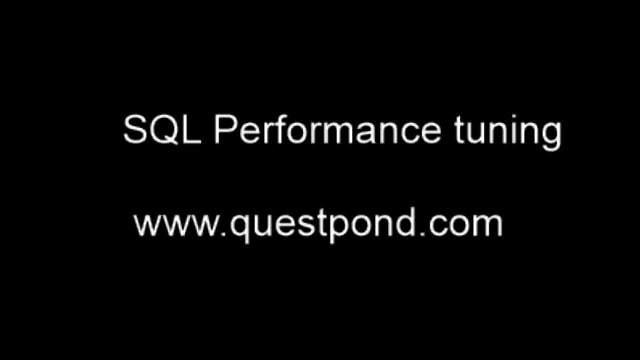 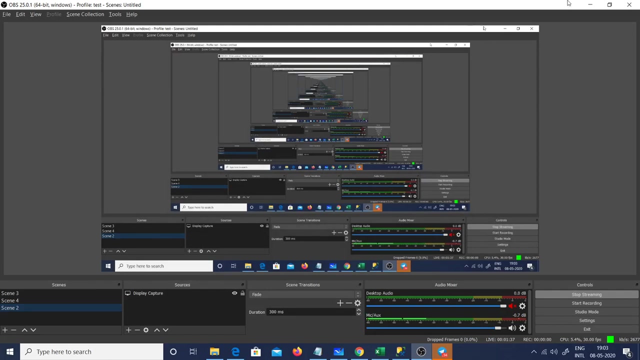 confirms that people can hear my voice In this SQL Performance Tuning. what is my today's goal? what is my today's agenda? So, very quickly, I am going to go and share my screen. So today let me focus on. so let me go to my white board out here and here it is. 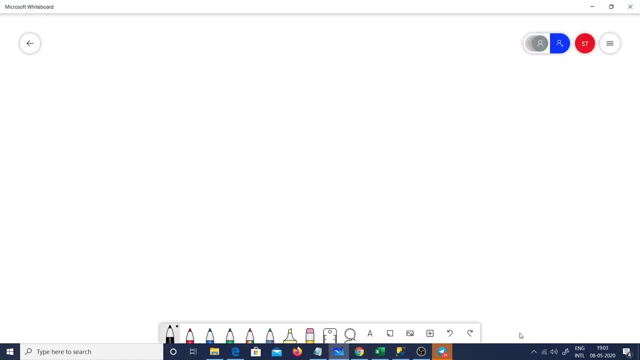 So now let's talk about, when you say performance tuning, I am assuming that everyone is new here to performance tuning, or at least you must have tried something at your end. but let me tell you that what exactly I do when I go to any database and if someone says something. 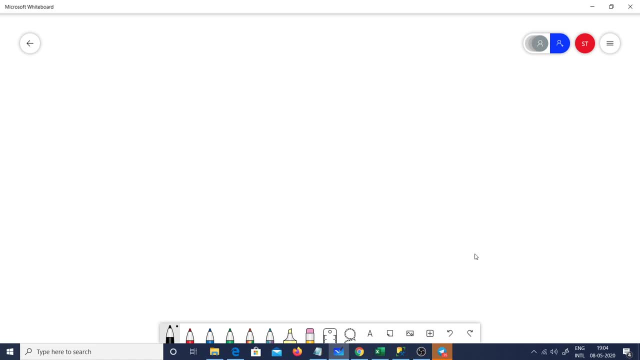 is running slow out there. Now there are two situations out here. The first is that when people know that which SQL is running slow. So situation number one: you know, like people know which SQL is running slow, right. and situation number two: people are not aware of which SQL. 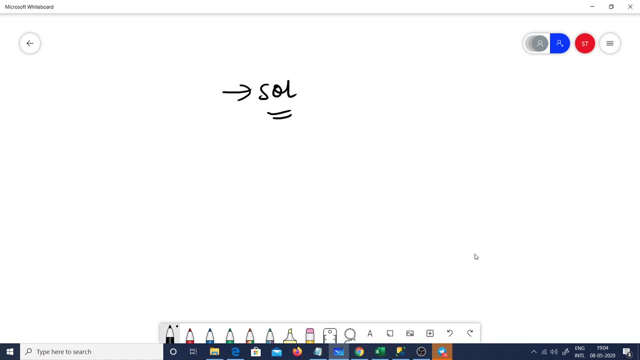 is running slow. what is running slow so must be. they have an idea that this is the screen. from this screen, whenever we click on the buttons, the SQL server becomes slow, right? So one is that you know exactly which SQL is running slow, and let me tell you that developers 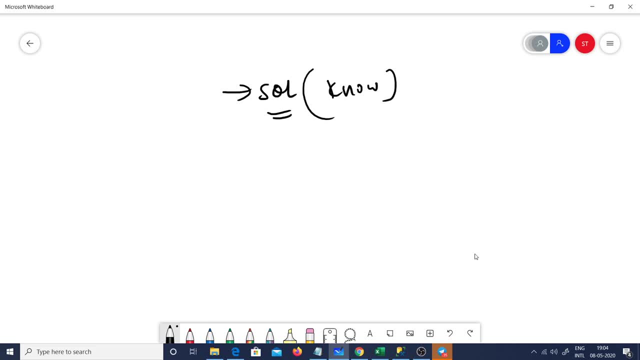 know everything. Developers have an idea that why it is running slow, right. and the second situation is: you know where you are not really aware of right. So now let's start with the second situation. you know where you are not aware of which SQL is running slow. 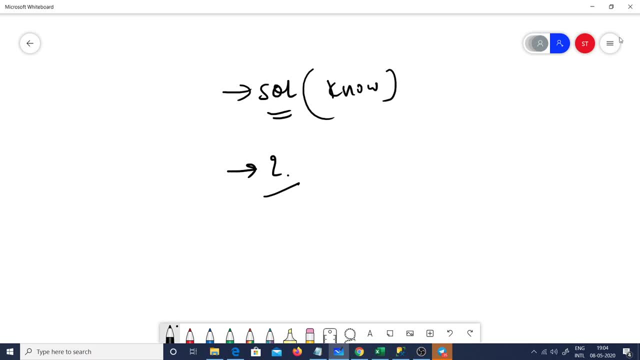 there are lots of SQL which is getting fired on your database, right? So you know. you can then divide your performance tuning phases into two parts. The first is the hunting phase. I will say the hunting phase, you know, saying that okay, like can I go and see you know which? 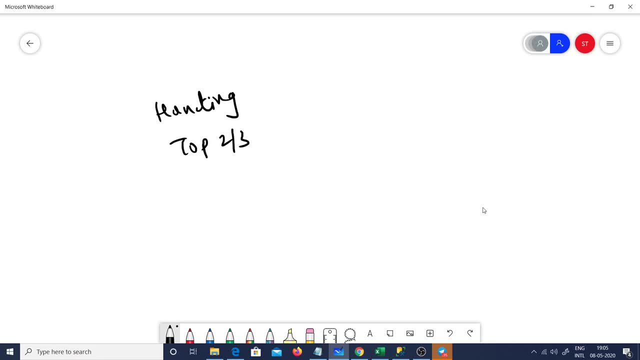 are? which are those top two or three SQLs, or which is that one SQL which is running the most slow of all of them right? And once you hunt you know what which the SQL is right must be. the other part would be to go and look at the query plan, look at the index, you know. so would be go and go more. 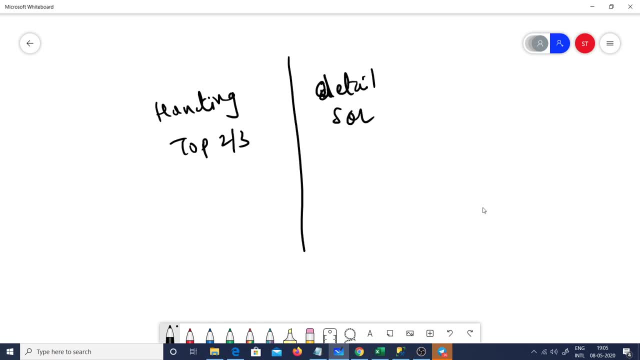 detailed into that SQL right. So this is one section. I am sorry, this is one section. you know wherein this is more on the SQL level. so you know more on the level. you know where you say that the developer has not written the joins properly, he has not set the indexes. 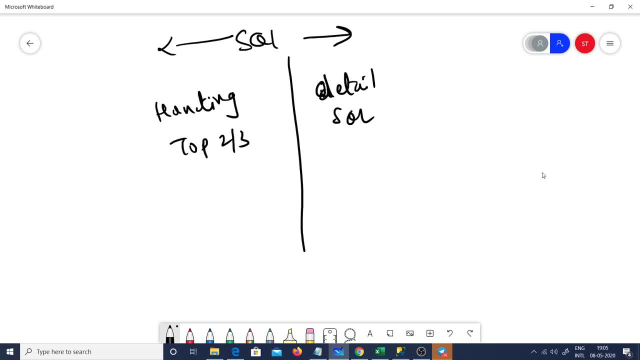 properly. The developer has, you know what you call- done a big loop or used a cursor right. So this is more you want to hunt. you know that is the code of the problem. Now in SQL server one, there can be a code problem. that means your T-SQL can be bad, the SQL which is written. 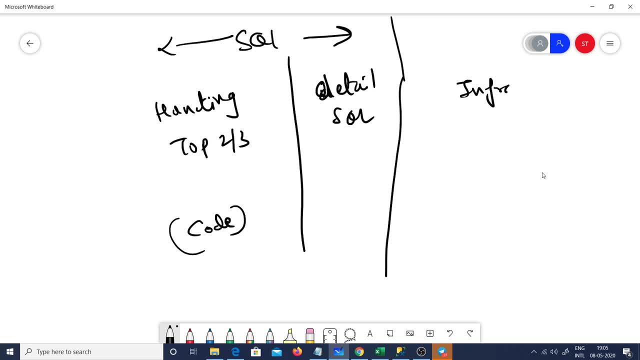 is bad. The second is infrastructure. Infrastructure means what the SQL is not defragmented, so there is fragmentation issues. SQL server indexes are not created proper clustered indexes, non-clustered indexes, those are not created proper appropriate primary keys are not set, and so on. 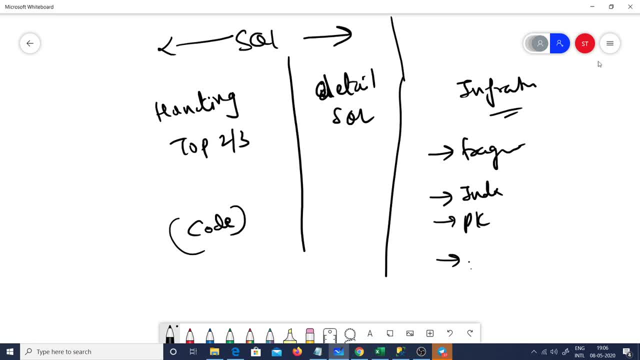 There are other infrastructure issues. there can be two broader issues. when you say that you have a performance tuning issue, there can be two broader issues. one is the code problem, the SQL problem. the another one is the infrastructure problem. Today I will only focus on only the code. let me not focus on infrastructure. 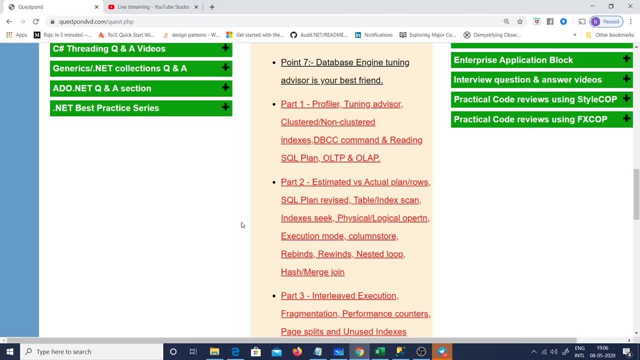 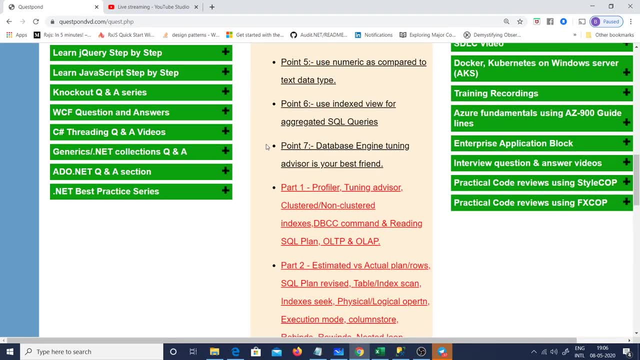 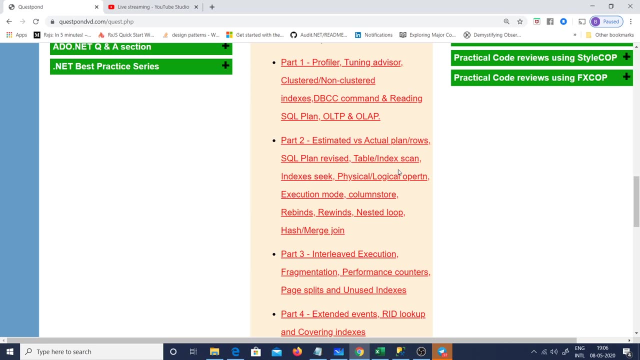 Just quickly, everyone, I remember that in our quest pond we had this long lecture of SQL performance tuning, which we had done in the previous month, where we talked about how to use the tuning advisor, how to go and see the table, scan, index scan, column store, indexes. 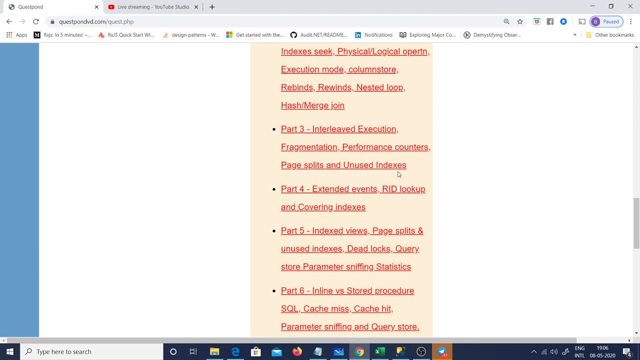 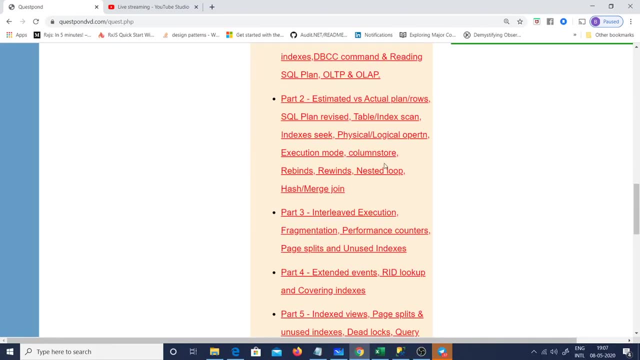 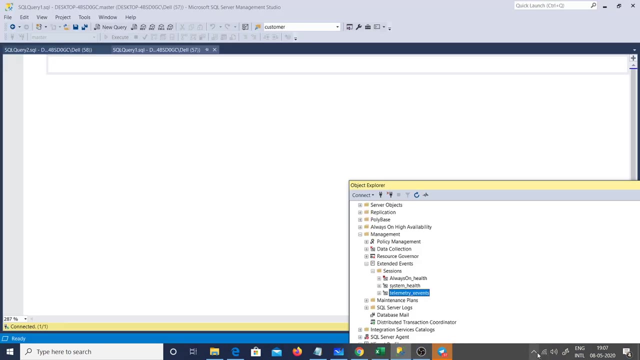 interleaved execution, which is the new one, performance counters, page splits, extended events, RID lookup. So when you say that really you want to do performance tuning, there are lots of topics out there, but today my goal out here is to first talk about how to go and hunt, which? 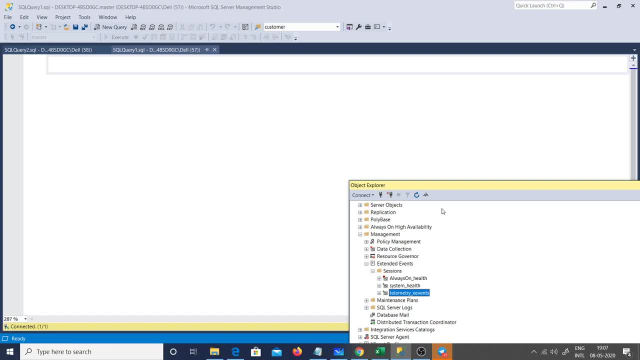 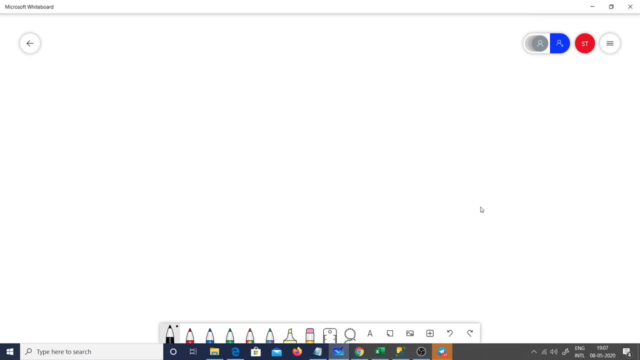 of my SQLs are not doing good. Now for hunting part, or to go and to listen to which of your SQL server are not doing good or what is happening with the database. there are lots of tools given by SQL server. Some people use the profiler. that is one tool. 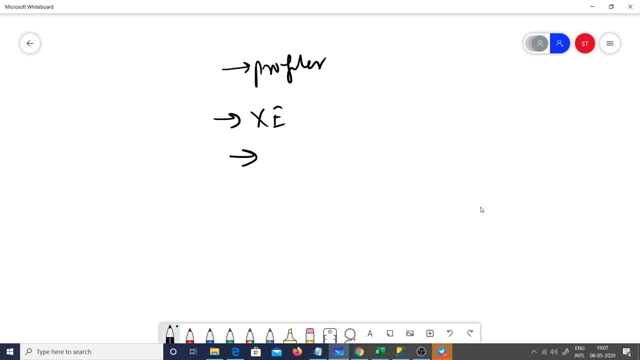 You can use the extended events, you can use the query store and there are so many other things provided. Now this profiler is becoming outdated, or I will say rather, they have decided that it is going to be obsolete. and second, one of the things to remember about profiler is that 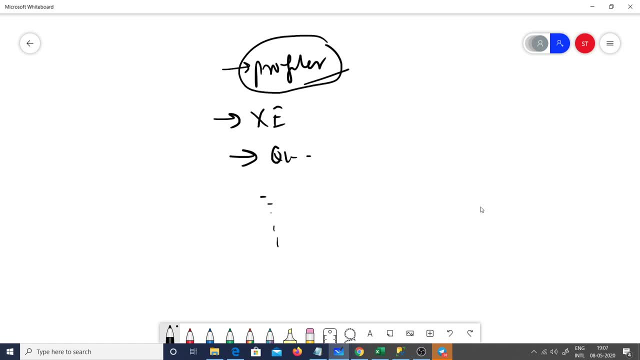 if you go and run the profiler on production, you can have problems. Why? Because the profiler goes and tries to block things, takes metrics and so on. Remember When you say that you want to go and hear something which of your SQL is going slow. 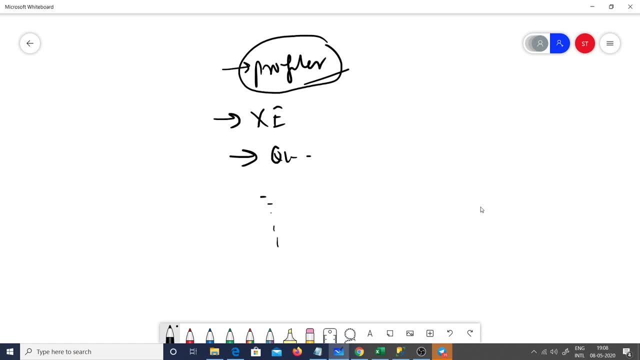 that means that this will have some hit on listening, some hit on your SQL getting executed, So you have to be very careful when you are executing these things on production. Another one which I like is the extended events. Extended events are like more lightweight. 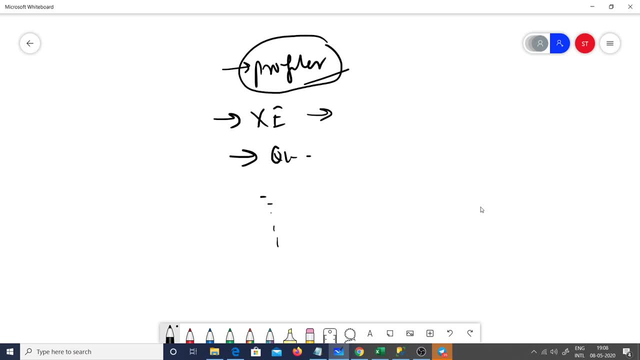 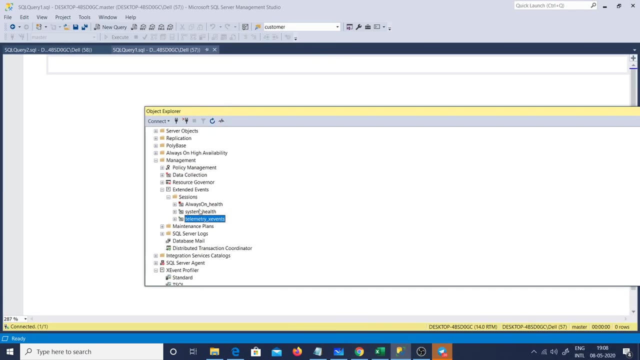 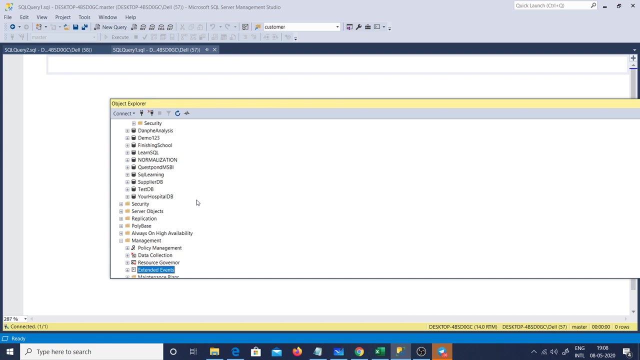 than profiler. They can be created easily. they are more powerful in the sense there are lots of more metrics which you can capture. Let me go out here and create a session. out here You can see my SQL Server. so let's go and find out which are my top 2 SQLs which are running slow, or the top 1 SQL which is 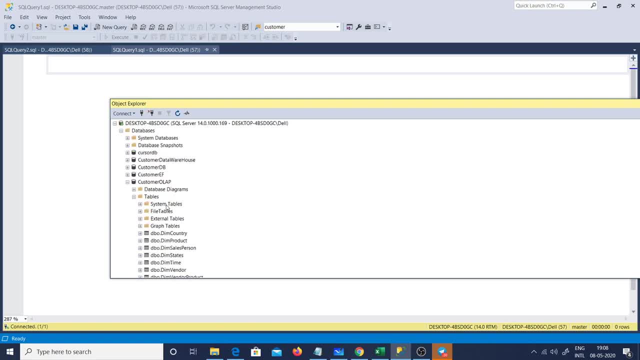 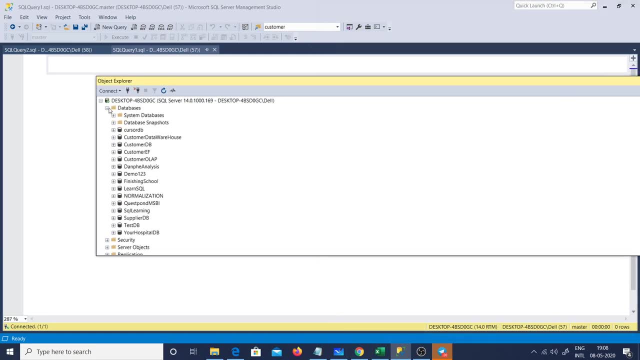 running slow. We can see in the SQL Server management out here. so you can see this is the whole SQL Server Object Explorer. In that you can see, see down below there is something called as a management folder. So I will go here to the extended events and let me go and start hearing to those events. So, extended events. 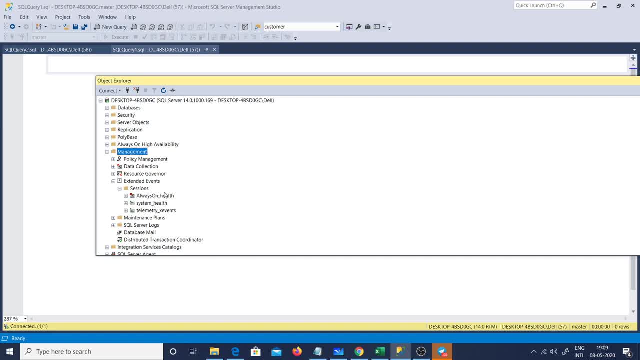 are nothing but events which are fired on SQL server. So, for example, somebody is executing an SQL, somebody is going and trying to acquire a lock, or somebody is going and dropping a database, So it goes and it listens to events and then in those events there are lots of 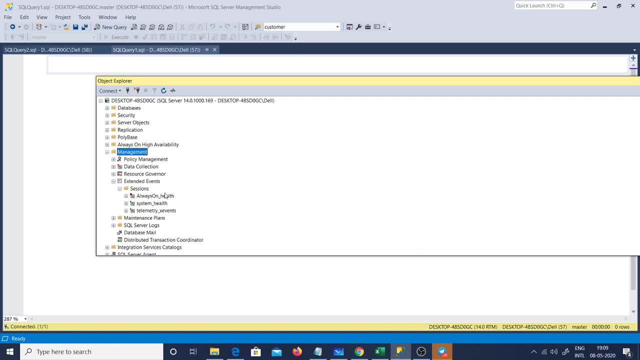 properties that time taken and is he using indexes? is he using clustered indexes, non clustered indexes? So there are lots of things out there. let me just quickly go and exit from all this which you can capture. So I am going to go and create a new session. so 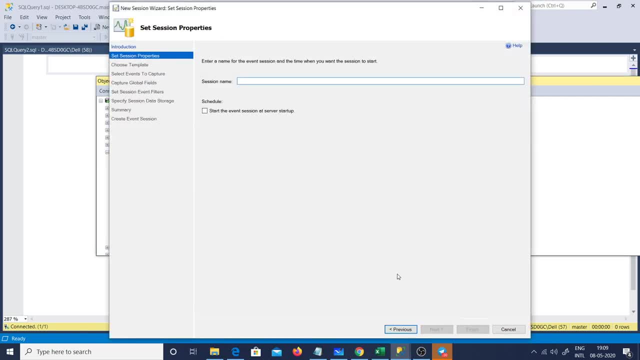 this is how, when you use extended events. So remember, this is phase one: hunting, hunting. you know where the problem is, So I will say that, okay, top bad SQL. So top bad SQL means SQLs who take the most time to execute. I can use an existing template In the existing 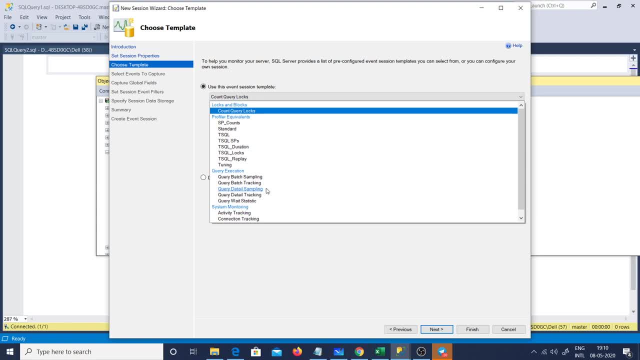 template. you can see lots of things out here, but we are more interested in the duration. Are you interested only in locks? Are you interested in only connections? Connections have opened and so on. Are you interested in the wait stats? Wait stats means when your 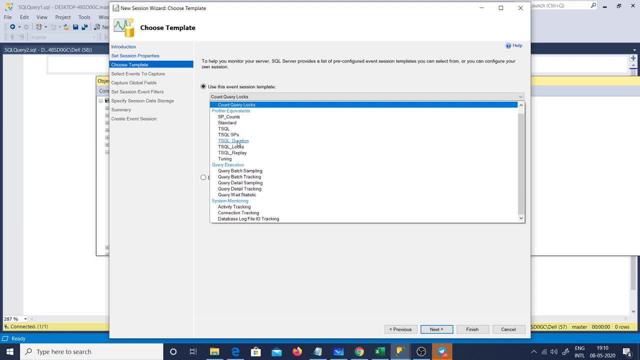 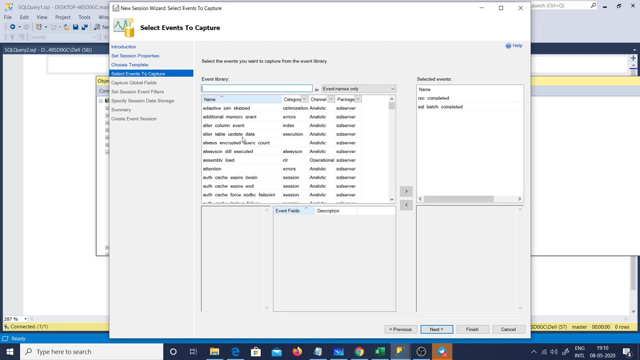 SQL was waiting and then when it started running- At this moment my interest is duration. I want to just know that which of my SQL are consuming high time. Now you can see the next event he says is that: do you want to go and add some more events? 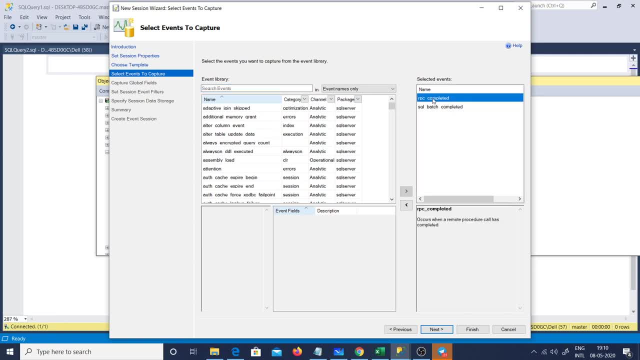 You can see at the right hand side. he has said here that these are the selected ones. like you will come to know when your remote procedure call has been completed and SQL batch has been completed. I am okay with that. I also want the start. Can we just try to take the start Also, probably? 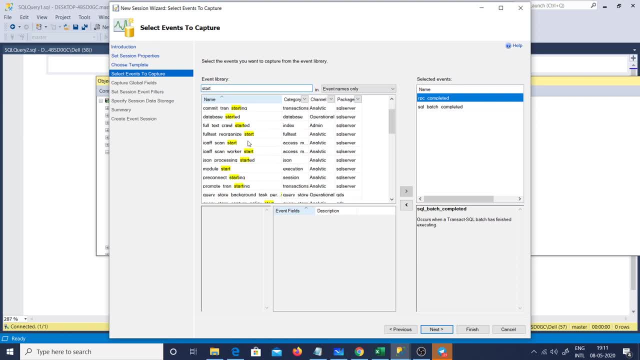 I am not sure, but even I would like to go and take the start. Let us not take the start because even if you look at this SQL batch completed, in this SQL batch completed also, we have duration. What I was thinking is that: do I need to go? 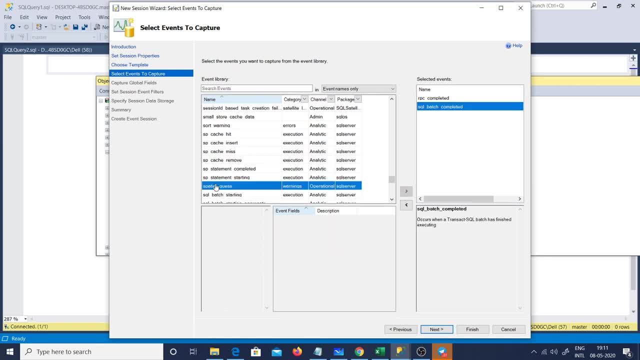 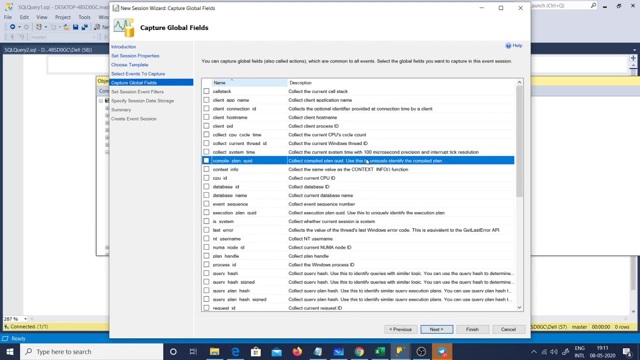 and take the SQL batch started and the SQL batch completed. I don't have to. What I can do is in this SQL batch completed itself. I have the duration and the duration is more than enough. Let me take that SQL batch completed. that is the event, and here it is. he says that these 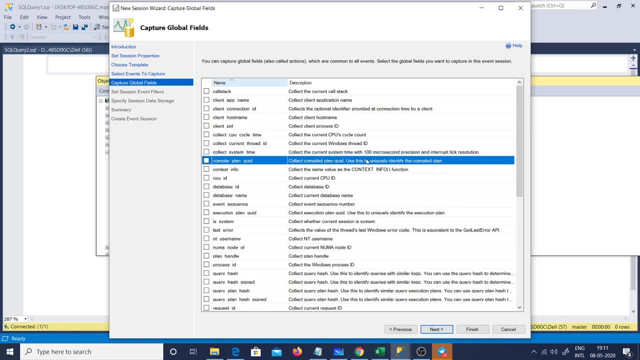 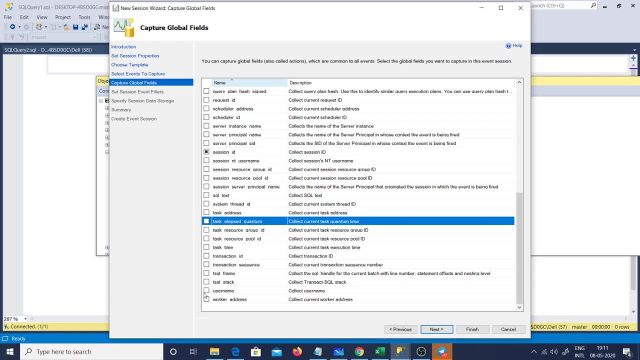 are the global fields. Do you want to hear something extra? Do you want to capture something extra? For example, one of the things I would like to really capture out is the user name in who executed this stored procedure or executed this SQL Next. do you want to go and update? 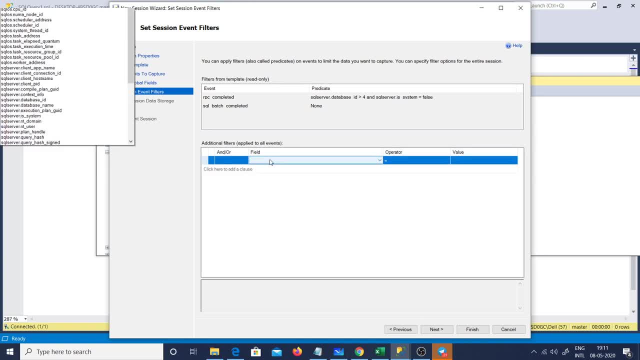 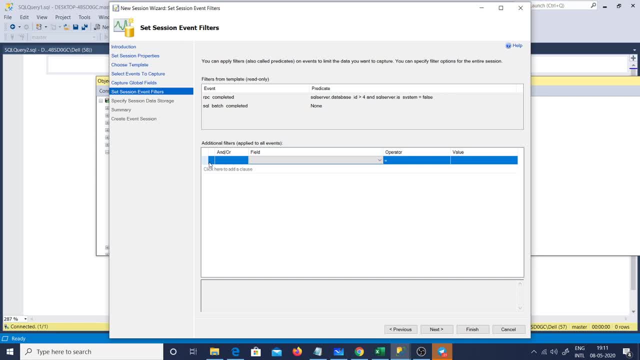 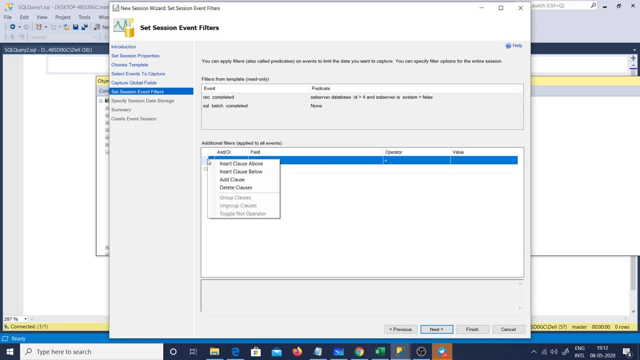 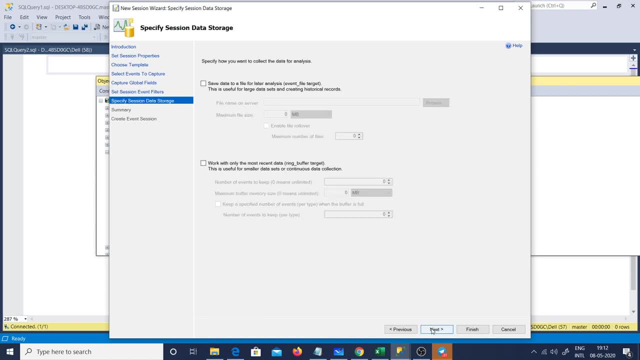 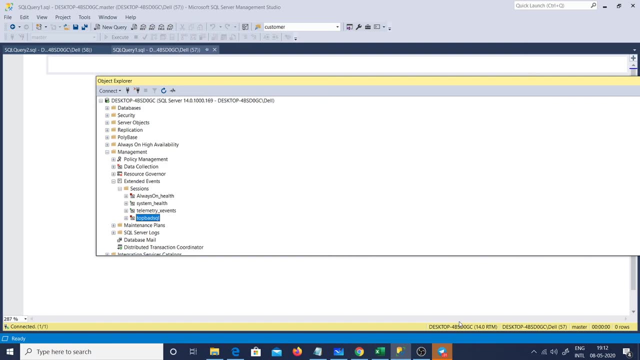 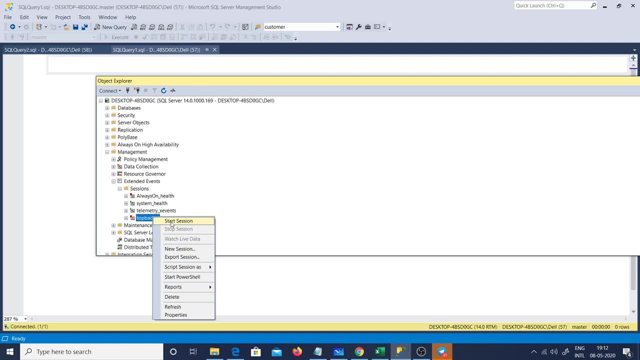 top bad SQL and I can go and I can start the session. start session means now it has started hearing to your database. you know, and you can now go ahead and see that you know which of your SQLs are running slow right. So, for example, now you can see I have a customer OLAP out here. don't worry too much about the. 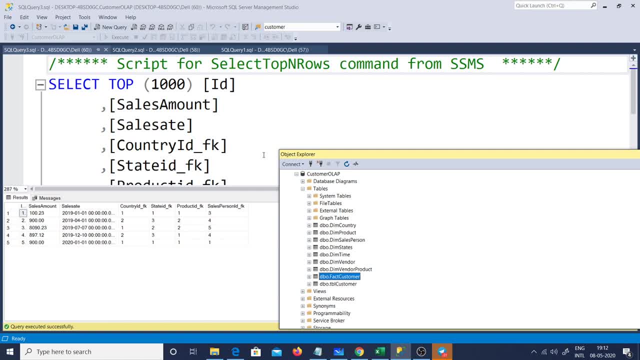 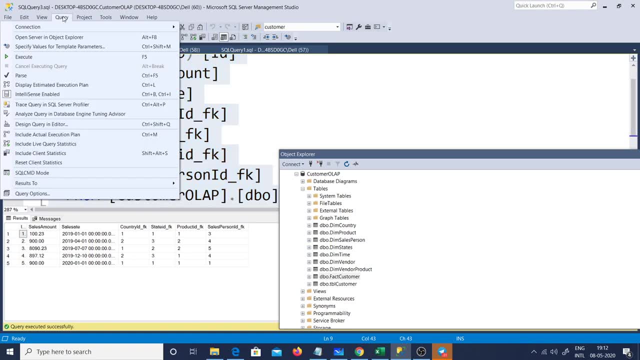 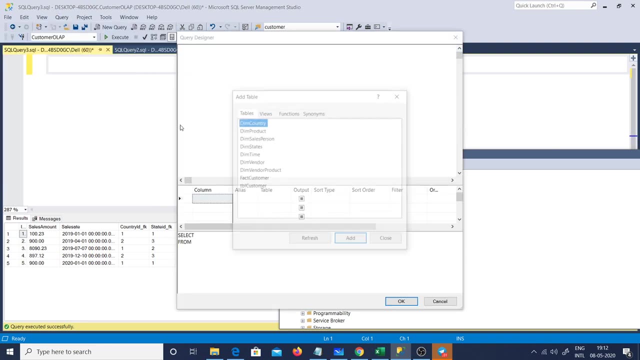 database at this moment. let me go here and let us take this SQL must be, must be. let me, let me go ahead and let me. how about going and taking? let me make some joins. you know, because when you talk about SQLs, you know some joins are. you would like to have some. 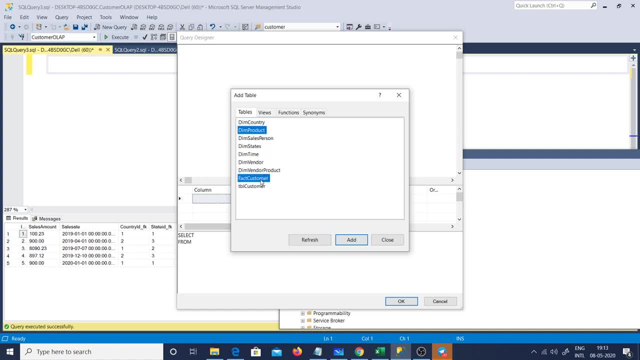 joins and get some more insight right, So you can see a dim product with fact. customer, don't worry, you know what is there in this tables. Don't worry too much at this moment in vendor right. so this is actually the sales and this is the vendor for the sales and this is the product. you know, nothing else. okay, and the 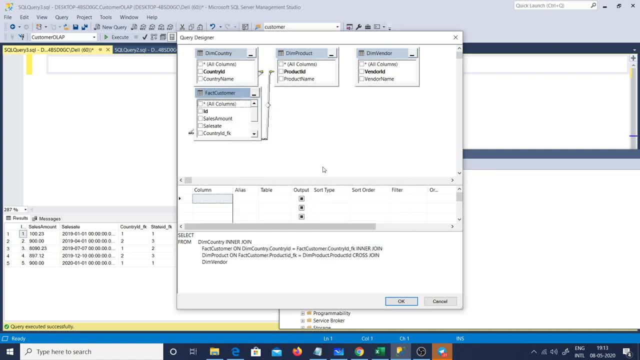 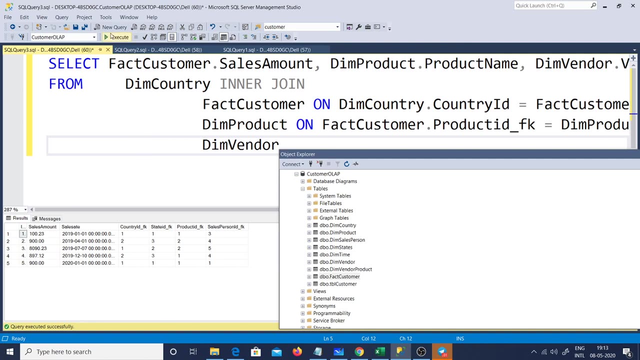 country where the sales is. so I don't want to write joins in this evening at this moment. so here it is: sales amount from here, product name from here, vendor name from here and country name from here. so I have just taken a inner join SQL out here, right? 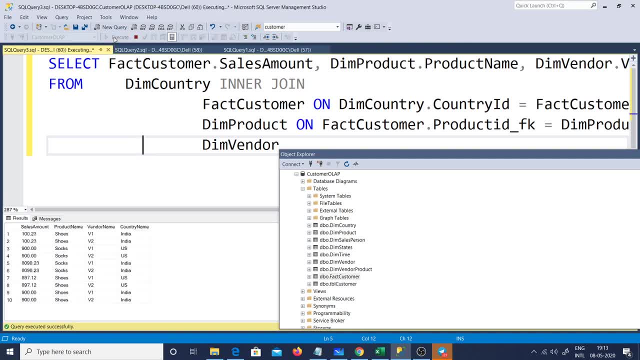 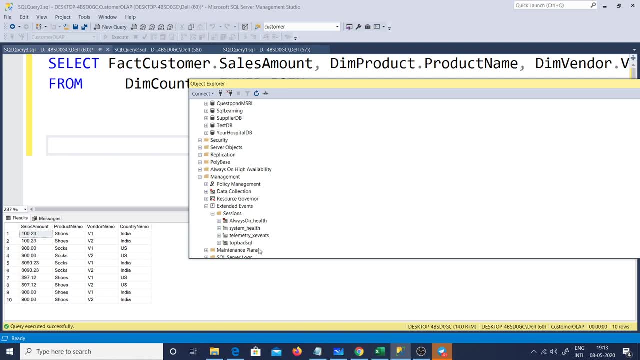 And I can execute this. I can execute it couple of times, right, so you can see I have executed here. now what will happen is, if you go now to your session, your session is still hearing it, right. so you can go to your session out here and say that, okay, can you, okay, you can. 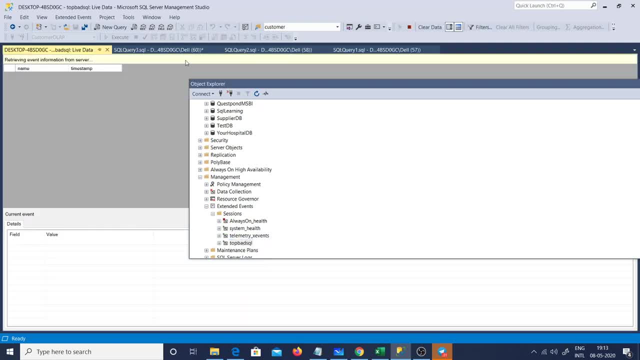 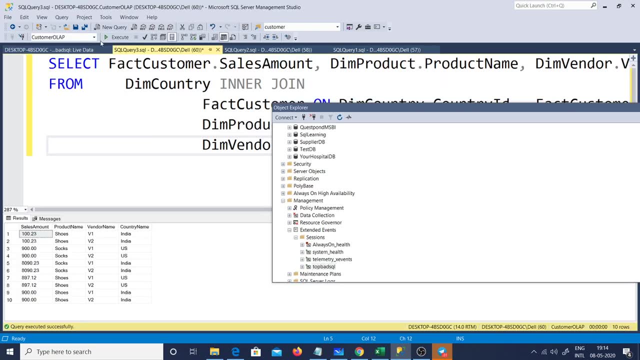 go and you can watch live data. you can see, I am going to go and watch live data out here. you can also go and see this live data afterwards now, definitely so. let us go and execute this. so I am going to go and execute this, and, and once I have executed out here, it should show. 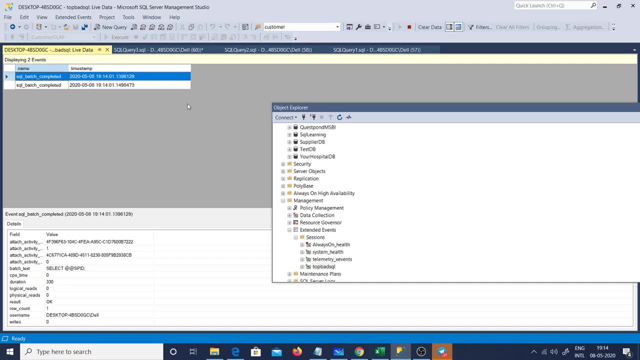 out here. You can see here. SQL must be here. SQL must be here. SQL batch completed. now, definitely, you know I cannot make out, you know which of my SQL has been executed, right, so I would like to see the text, the SQL text, so I can go out. 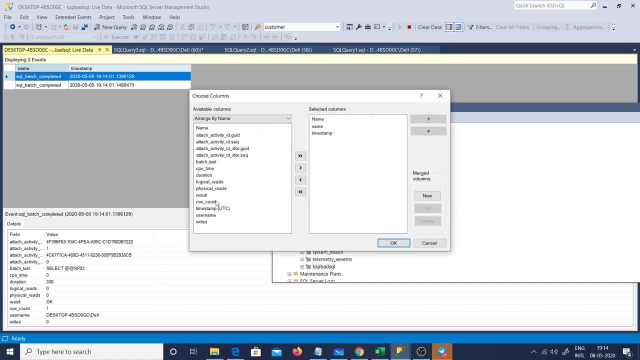 here and I can say: choose a column and let us go and choose the batch text. so the batch text, you know. with this at least I will come to know what kind of SQL has been executed. so you can see here and also the time. yes, I would like to also get the time you can. 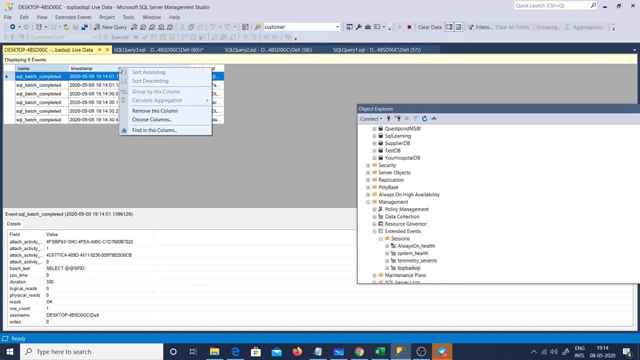 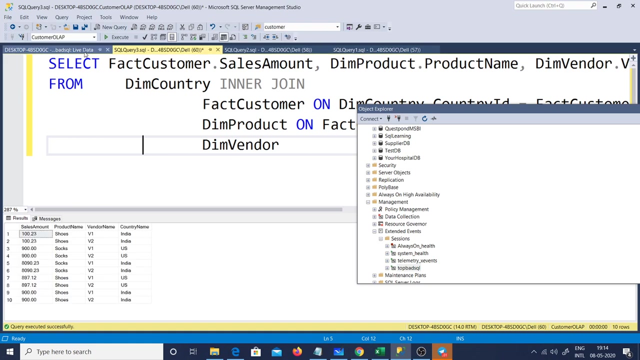 see there are some other SQLs also getting executed out there. Also, I want to get the duration duration. there is a duration out here, right, great, and let me sort this. let me sort descending what happened out here. okay, it is live still, so here it is, you know. so whenever I now fire any SQL anywhere in my, in my application or in my, 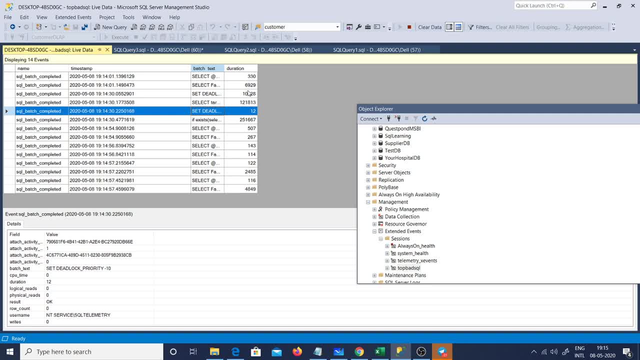 SQL management studio. it start getting logged out here and what I can do is I can later on go and stop this session. I do not have to hear this session For a lot of time. so what you can do is you can go and do. sampling must be in between. 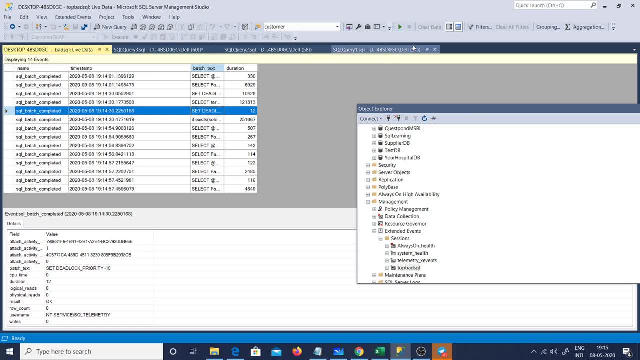 of the light production time. light production time means when the production is not so heavy. even if something happens, you can still like recover back, and so on. right, so you can go and you can run this and you can get an fair idea, and then afterwards you can go and start. 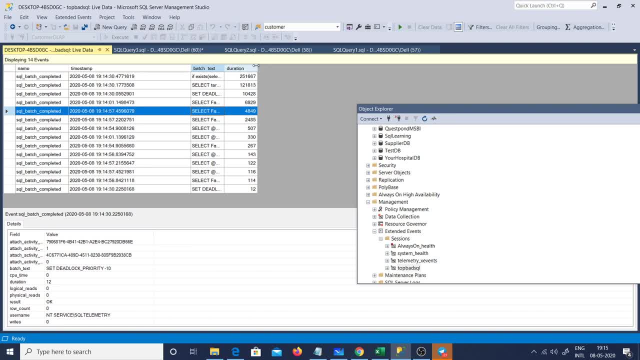 doing lot of things, you know. for example, you can say sort descending, so now I see out here that this is a, is the, is the SQL which has taken a lot of time, and also you can see some other SQLs out here, right. So from this text I can now make out that which of my SQLs are my top four or five, which? 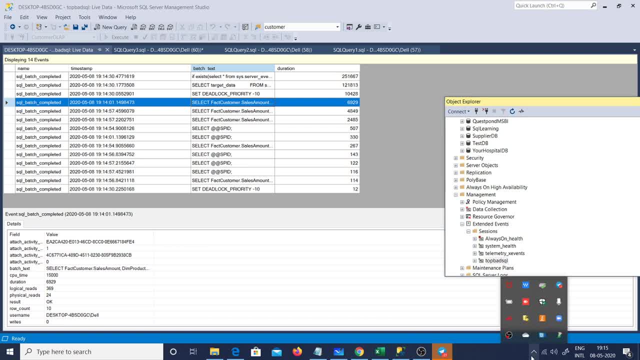 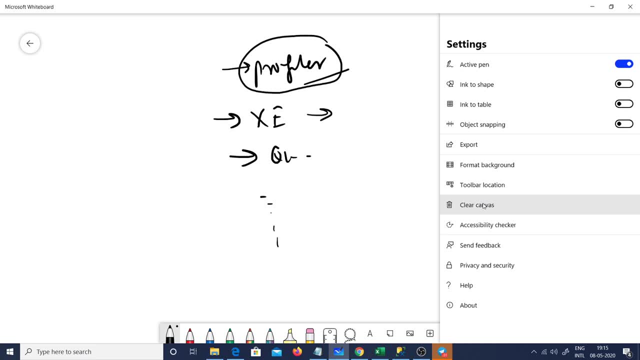 is running right. so the first part, which is very important, is to hunt. you know what the problem is, you know, so you know, think about it. you know logically what happens is. so think about how logically you will hunt a problem right. so first is, you would like to know where. 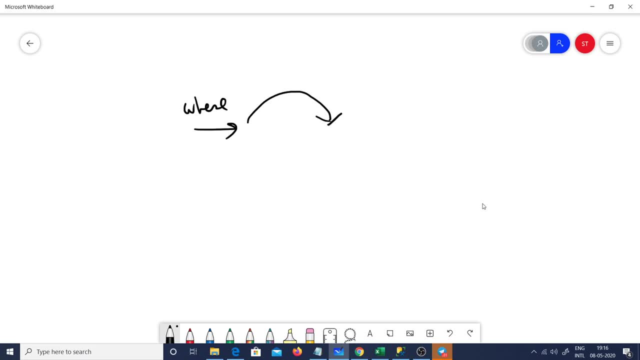 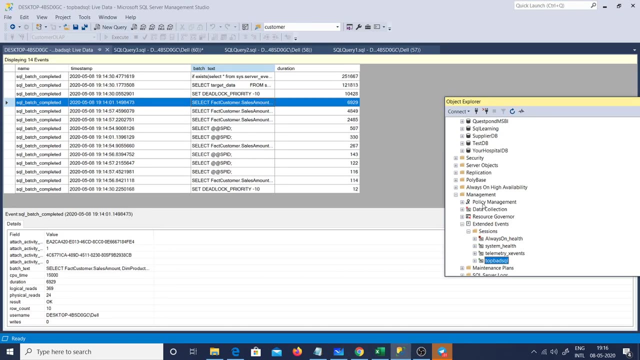 the problem is the hunting part. and then you would like to go more in depth and say that, okay, like So, this is the SQL, So what should I do for it? right? So this is the first part where the problem is right. So, guys, if you have any questions, what you can do is you can put down on the chat below. 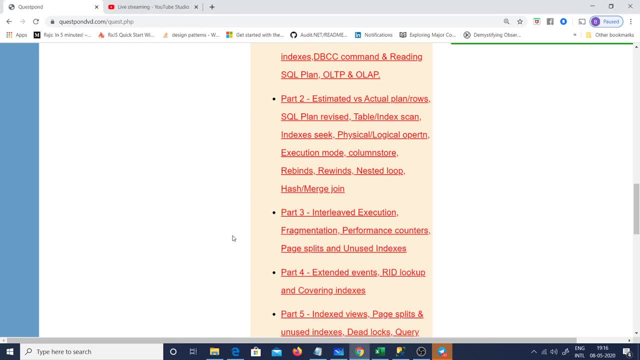 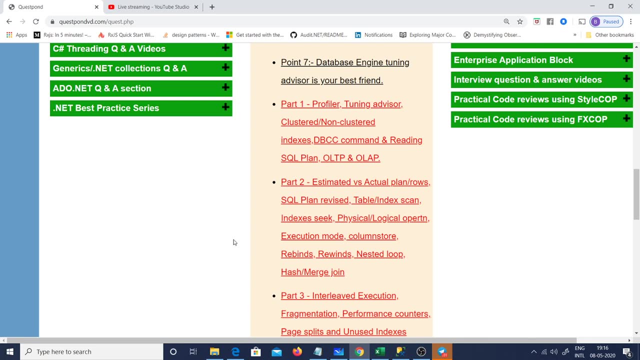 and very quickly again. I repeat: you know, when you talk about performance tuning, it is lot of things, it is not just this, right? So I would suggest you know that. read: I am not saying that you take my course, this is not an advertisement. I lied out there so. but the point is that I, you know, you should know. 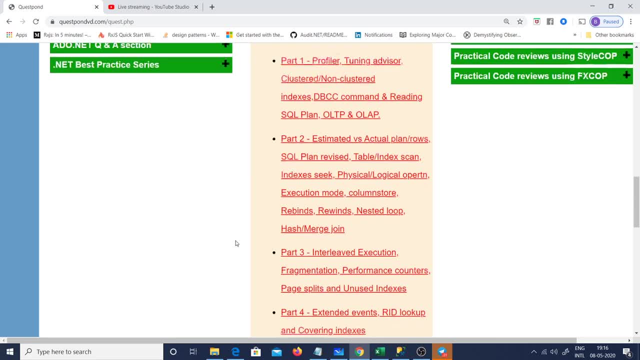 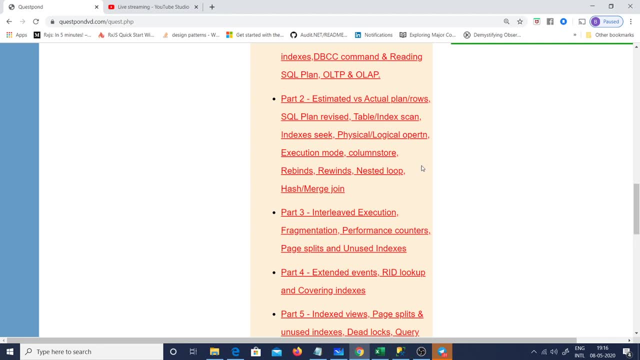 a lot of things you should know: performance, how to use the tuning wizard. you should know how to go and what is a column store. you should know what you mean by the physical operation, logical operation, index, scan, index, seek. how to use performance counters. again, performance counters are one of the ways of doing it. 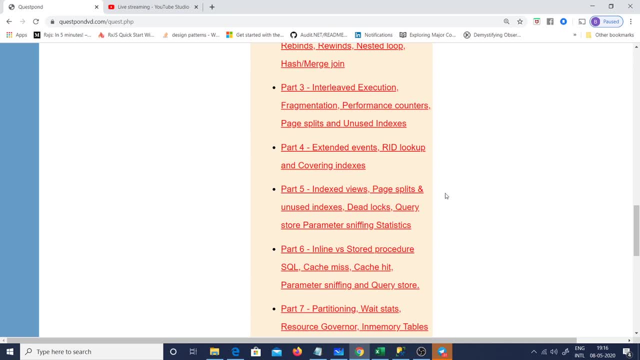 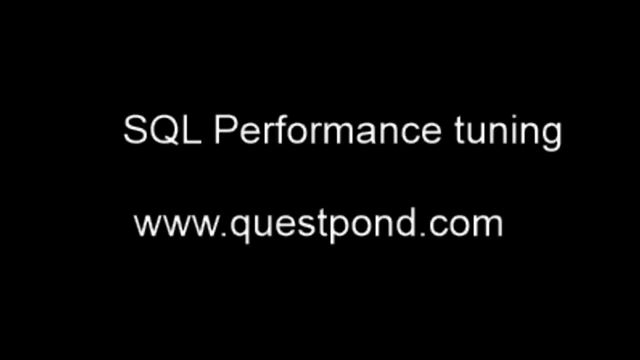 Rid lookup and in SQL 2019, if you see there are lots of more features. you know which they have given, for example, the SQL store and so on, right, so first thing, any questions on the SQL. Oh, you know how to go and hunt it, So I just showed one way of doing it. extended events. 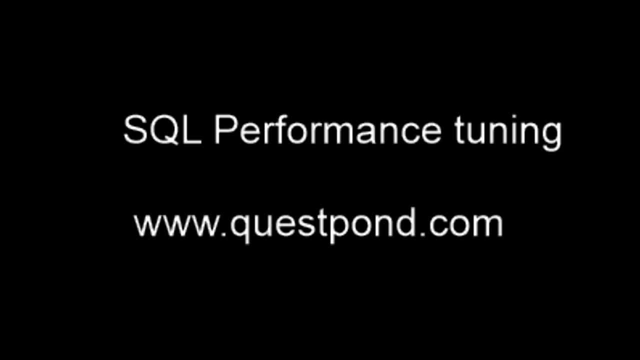 So let us see if there are any questions out there. Please zoom the screen. I am so sorry. I am so sorry for that. Okay, so wow that I should have done it. So my screen was not visible. that is so sad. I was there for 15 minutes. oh gosh, My screen was visible, or? 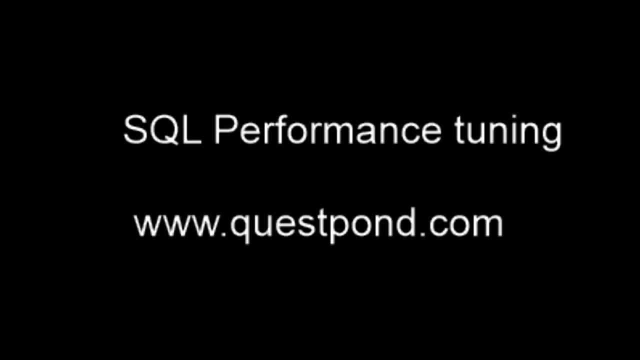 it was like. I am so sorry for it. That is sad to see. Okay, I just went out here to check. Okay, so let us see the questions please. Okay, so let us see the questions please. Okay, so let us see the questions please. 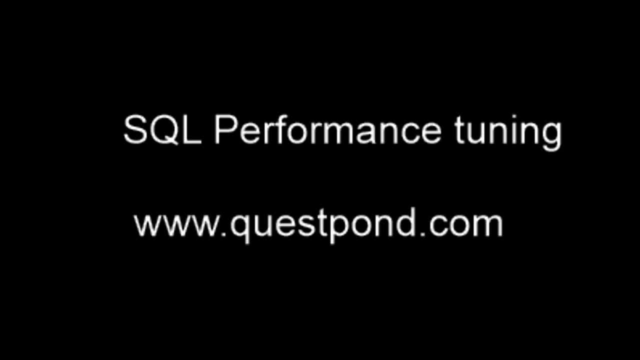 Agree, and I will put down the questions out here. I have completed how to go and hunt the SQL problem. So a question from Ravi. here we have an execution plan for a query. yes, that is right, and the execution plan for the query and execution plan are different. 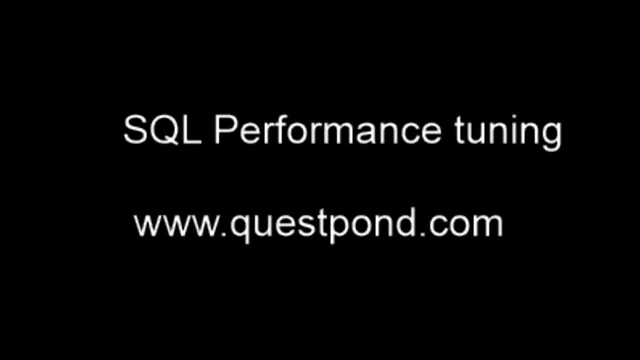 No, query is, these are sessions. yes, So, Ravi, these are sessions. these are extended event sessions. these are extended event sessions. yes, The session is different and execution execution plan is different. Execution plan is more in depth about the query. Will this? 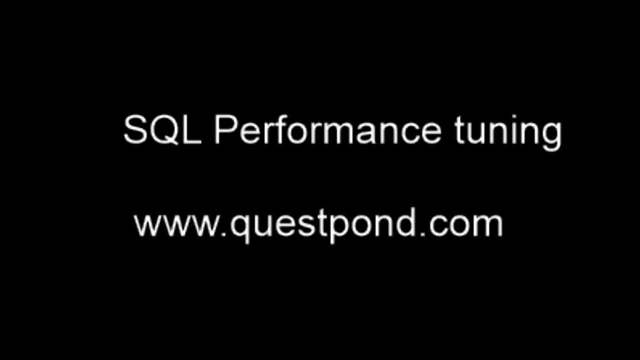 video be available on YouTube? Yes, absolutely, ma'am, it is all available on YouTube. If I got a message, MySQL server is having some issues before one week, how can I find that issue So over here? please note that if you have some issues, then you should have a history. 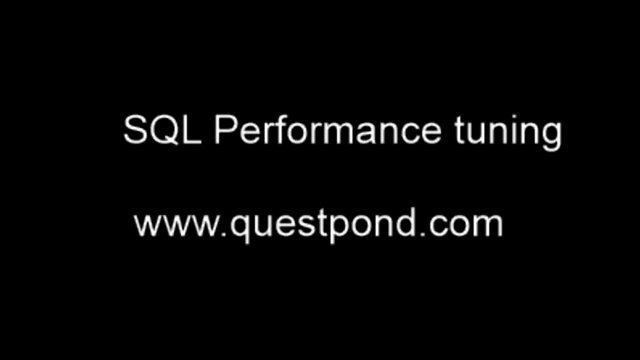 of it, For example, that if you have logged a session, if you have logged extended events, you can go through that, you can filter it, you can go and look into it. you know that was the time the problem was, locking the problem, and so on. If you don't have a history, 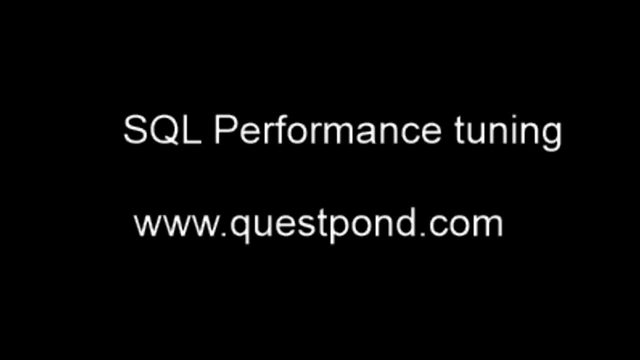 then it is very difficult. Only left mic is working. I mean the left earphone is working. Why is that? with everyone Left earphone is working. Profiler and session. so sessions, Abhijit. session means it is extended events, So that session is nothing, but it is extended. 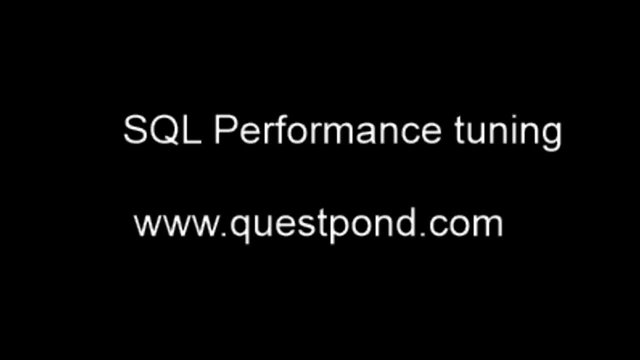 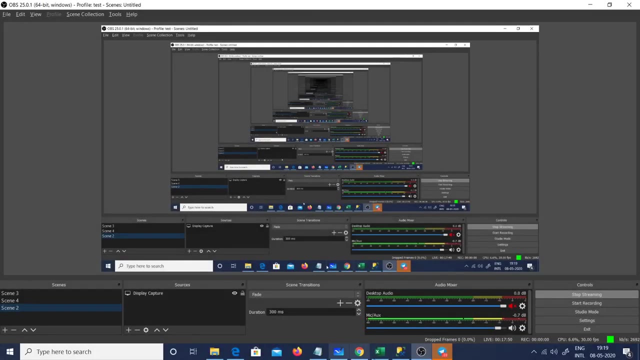 events, That is the right word to use. Profiler is different, extended events is different. So a good question from Vidya here. A profiler means. so if you look at profiler, I can just show you that Profiler is bit heavy. So I can see there is a question out here. what? 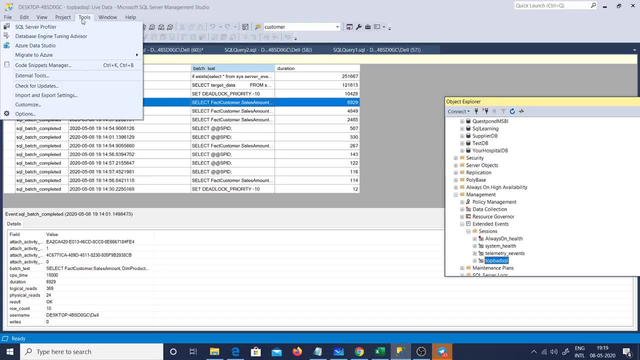 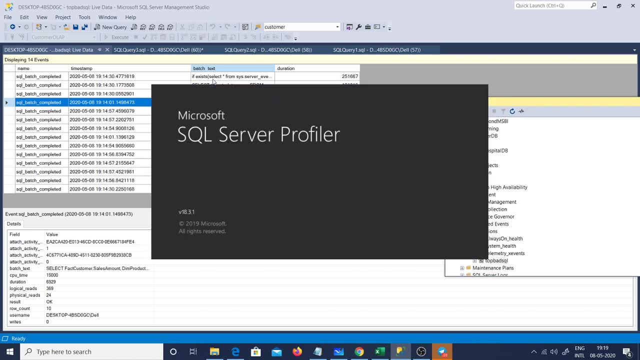 is a profiler. A profiler is again a tool. you can see here. this is an SQL server profiler on the screen So you can go to this SQL server profiler out here. This profiler is a tool you can see exactly here. there is a profiler and there is outfits in this perfiler. I mean. 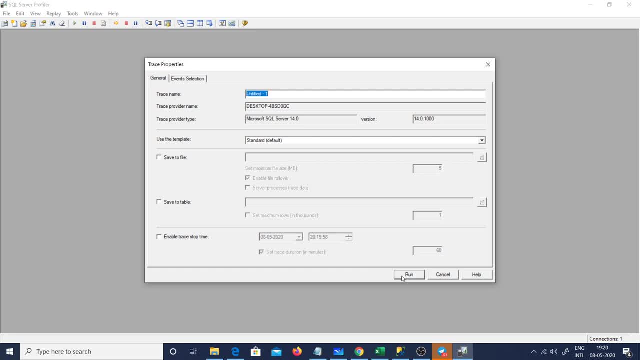 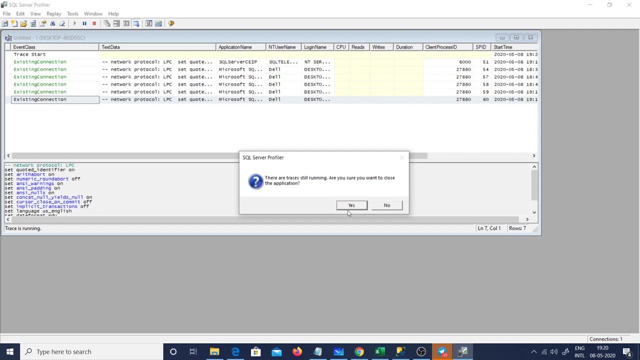 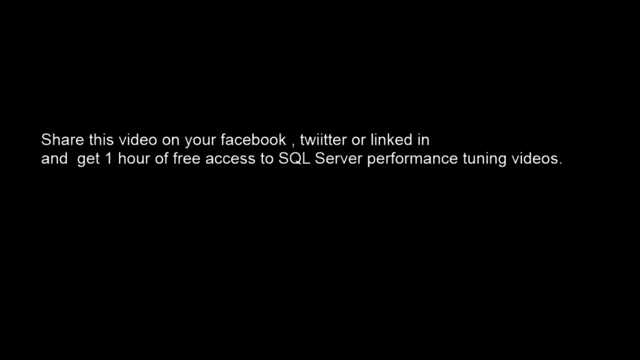 only default focusing on this screen being an iPhone, and they also show that a descent to cover a specific interface properly and that means that it shows this error shown very clearly. There is more führen in this Ki it. it just shows like a viewer river it. 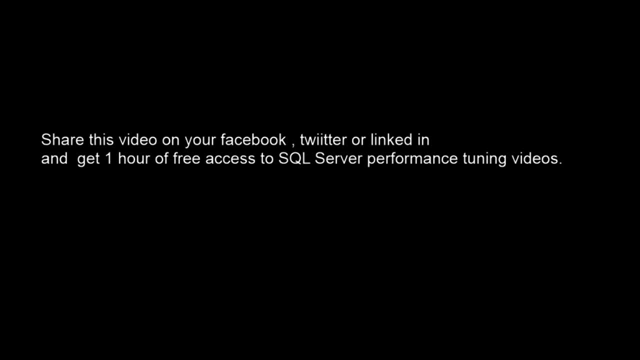 says hago Sounds very natural. I have it in Java and 365.. That's a good question from Tech Genius. Query execution first only takes more time. How to reduce that time? by using stored procedures. Most of the time when you say that a query 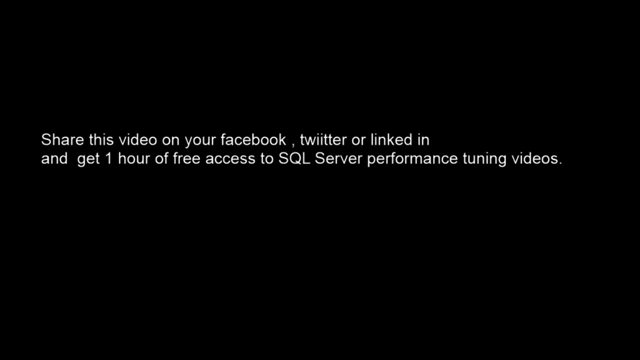 is taking time. first time that means it is creating a plan, So must be. what you can do is you can use stored procedures and just ensure that the plan is created only once, and then it should help out. There are two, three things which happens when you start. 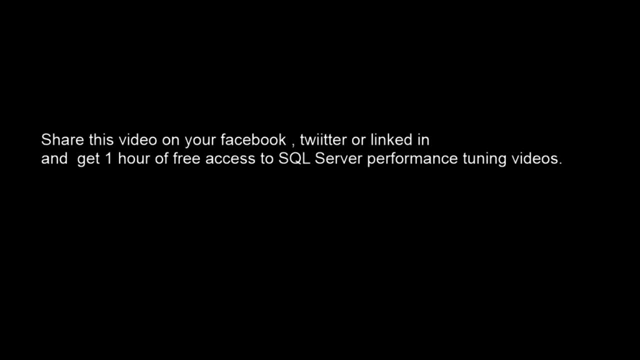 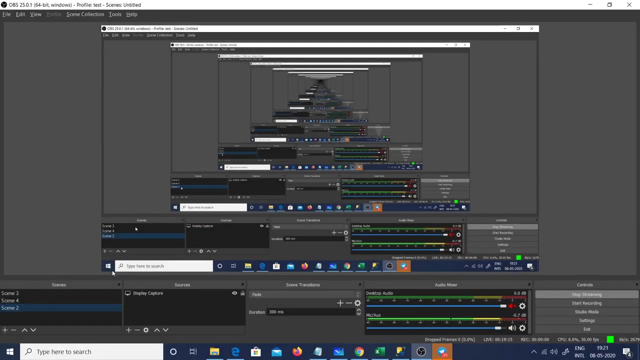 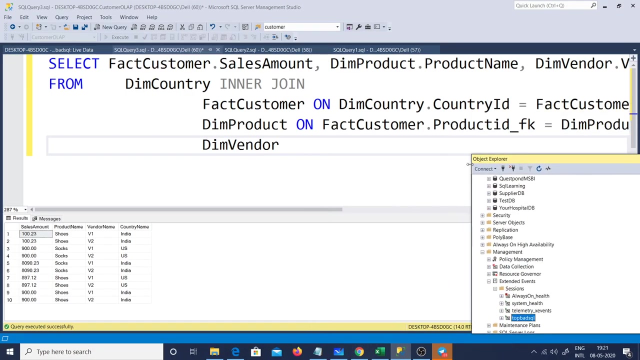 executing a query. One is there is some kind of memory which is needed- caching and so on, and second one is the SQL plan. With all this, we know that our SQL is now very much slow out there. Assume that this is the SQL which is very slow, and now we want to go here and we want to see the plan Reading. 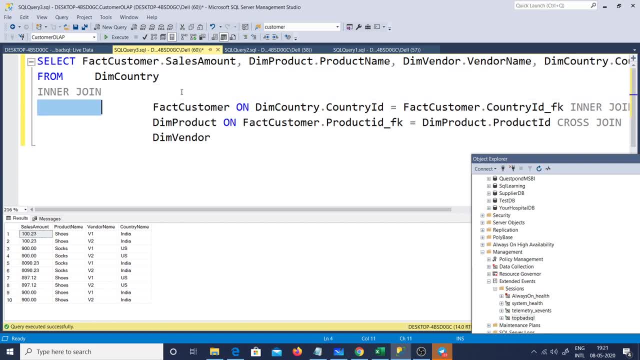 of the plan. this is the second step. Once we know this is the issue. Remember, today I will not be discussing about infrastructure issue. Infrastructure issue is again like one more issue which you should know. For example, is your fragmentation done or not? Is your indexes in place or not? So infrastructure: 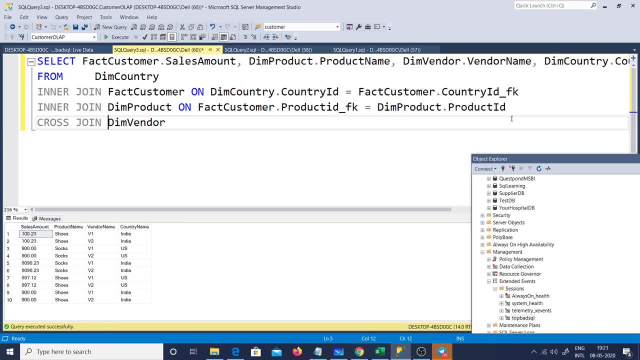 what you should do is you should create a kind of maintenance activity and tackle the infrastructure issue. Today I will not really go into infrastructure issue, So let us assume that this is the SQL which is running very slow and we want to go and see why it is running. 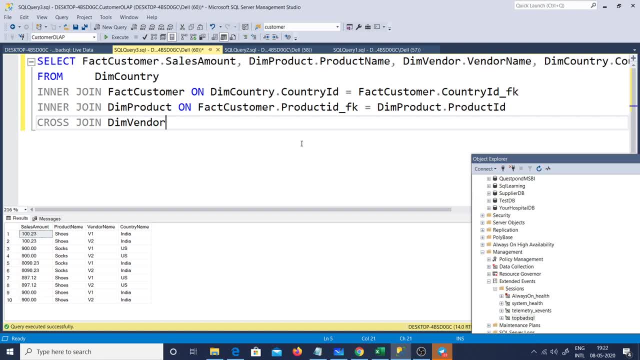 slow At this moment. I have just taken any SQL which is there on my database, but assume that this is running slow. So for that you know we can go and we can see something called as a plan, SQL plan. What exactly is an SQL plan? SQL plan is nothing, but it is a logic how that SQL will be executed. 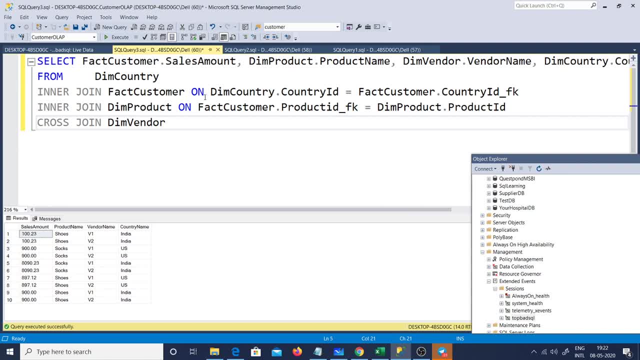 by SQL server. So, for example, over here, if he says that he wants to go and make a join with this country id and this foreign key, Will he go and loop row by row? Will he go and use an index? Will he go and merge them? 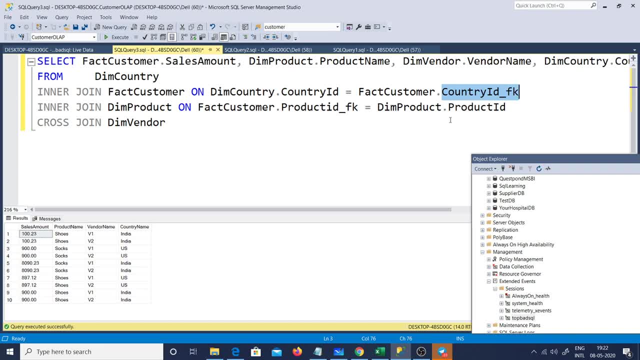 and do so. It is a logic. It tells that how SQL server will execute this SQL logic. So now you can see out here if you want to go and do the SQL plan, you can see out here. there is something called as this display: estimated execution plan. You can also say: 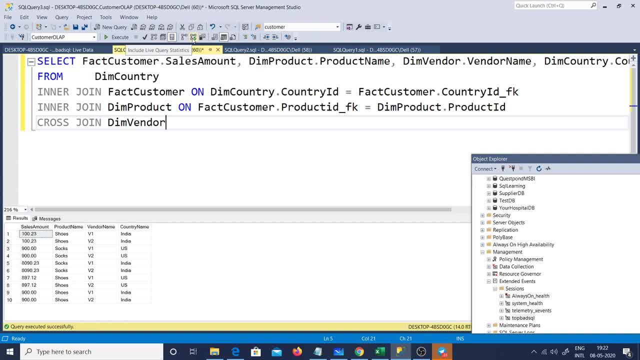 here display actual execution plan. There is something here called as live query statistics, So we have estimated- Estimated means- what It will go and it will not run SQL on your live database. It will go and look into your current statistics. what you have There is. 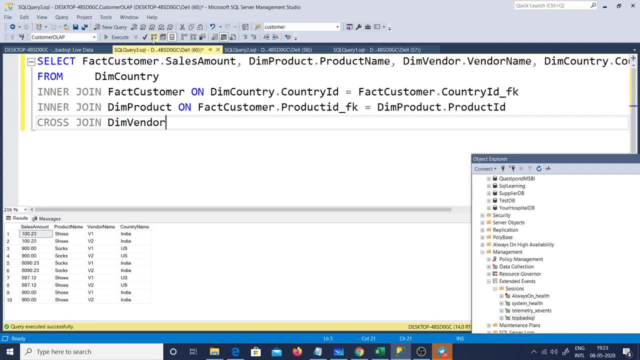 statistical database, also internalised 2-3 tables, which maintains the statistics. He will go and will not fire on the actual data and from whatever statistics you have from the past he will try to go and show you a plan. When you say actual huge database, I would say avoid. 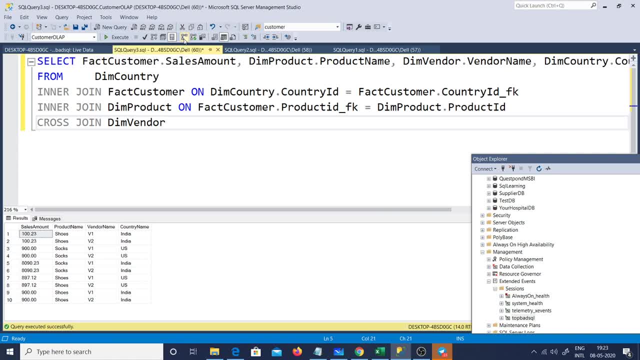 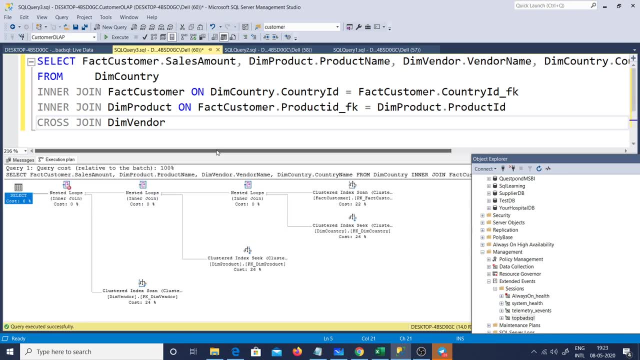 execution plan. you know, attach execution plan, actual execution plan, because that can really go and hamper your production, right? So let me go out here and let me click on the so you can see out here what I have done is I went here and I said: display execution plan. 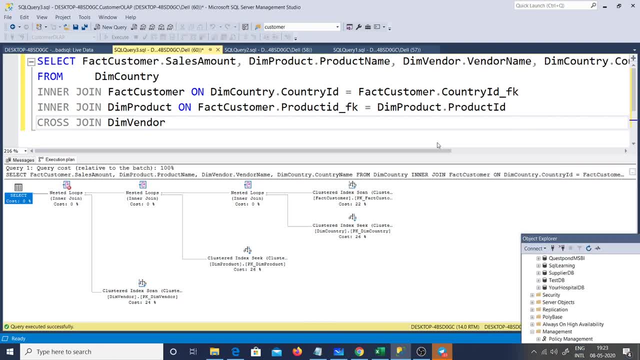 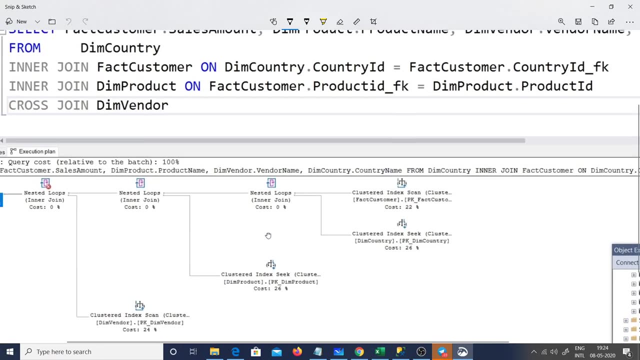 right, and there is my execution out. there must be. we can zoom so you can see this is my execution plan. I can zoom on that and let us try to understand some of those things around it. right? So that is the execution plan. at the top we have the SQL. Let me see. 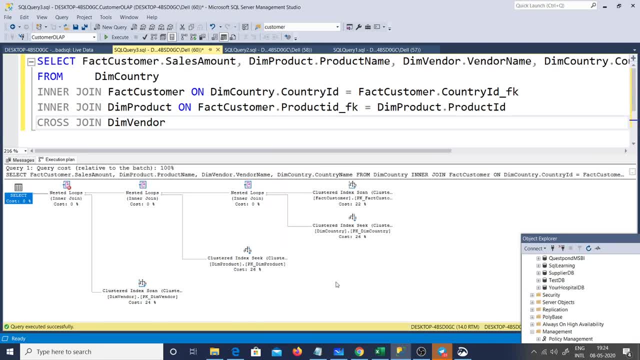 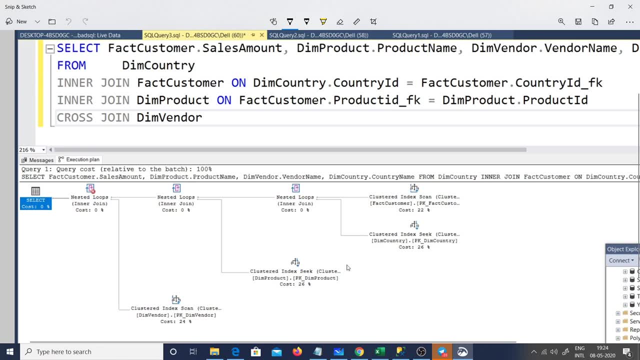 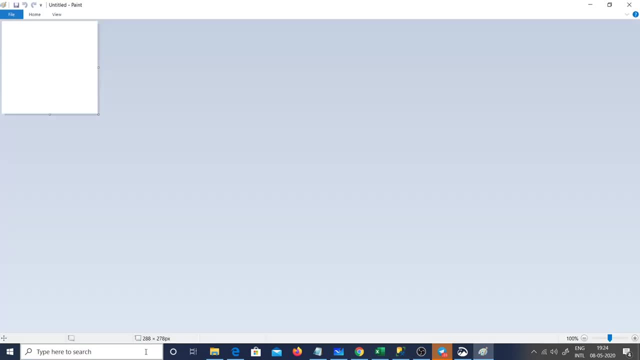 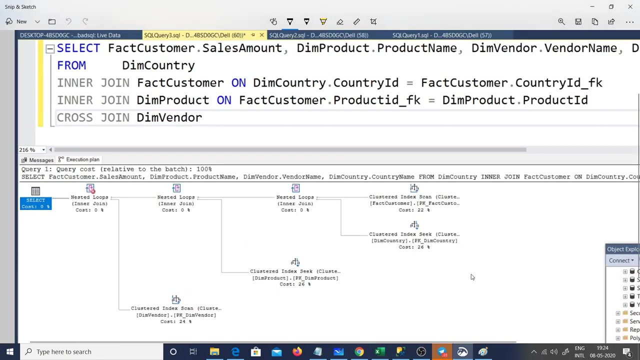 if I can. oh, I can't, okay, we will see this later on, right? So here it is. let me do like this, Let me function. Let me do this because I want to show even the. let me, let me take that pane off. I always 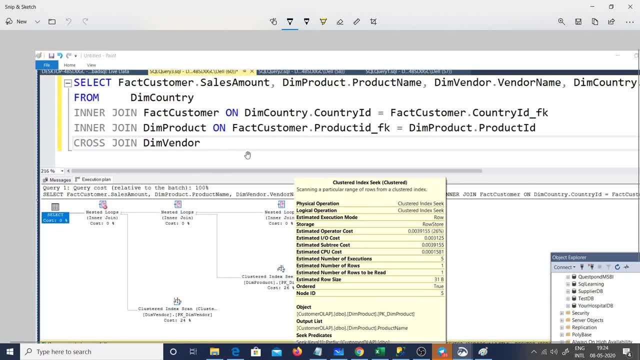 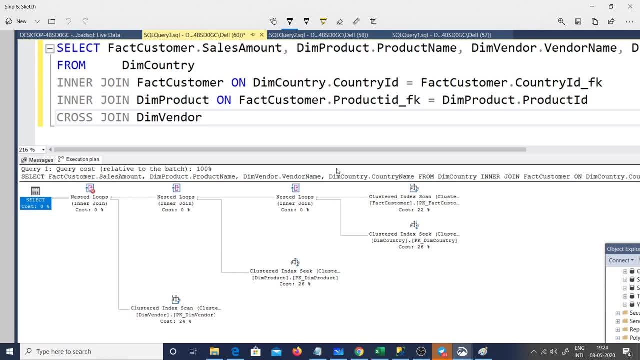 feel that you should write, you should draw, right, okay, So let me go here and then I will go there. So here it is. first thing, this is the execution plan out here. right, You can see I have I have two inner joints And I have one cross joint. So you can see inner joint out here. inner joint out here. 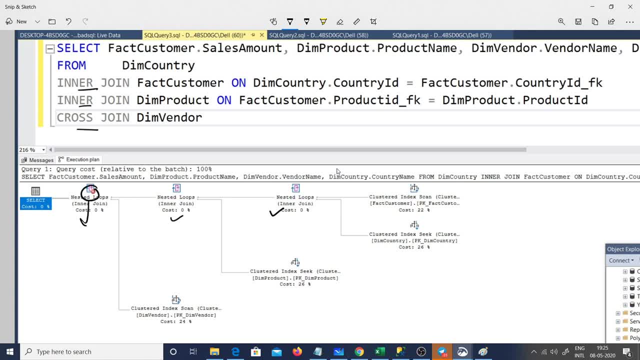 and this looks to be a cross joint. That's why it is showing a red color out here saying that that this is something terribly wrong out here. So SQL server is pointing me out there is some problem out here with that red sign. right, You can see that red sign out. 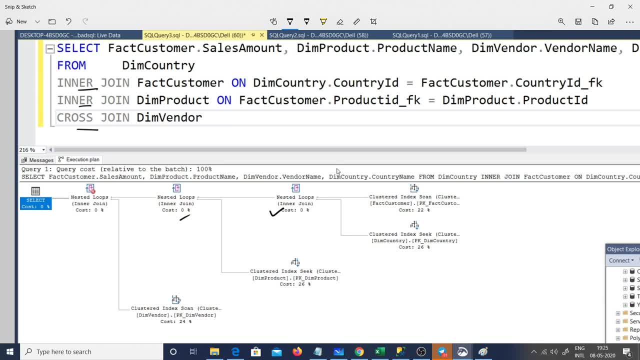 there, right, But you can see like: so I have joints and so here it is. you can see that here it says that this is so. that is one part. The second part is: you will see that there is a cost here twenty two percent, twenty six percent, and there is some kind of a cost twenty. 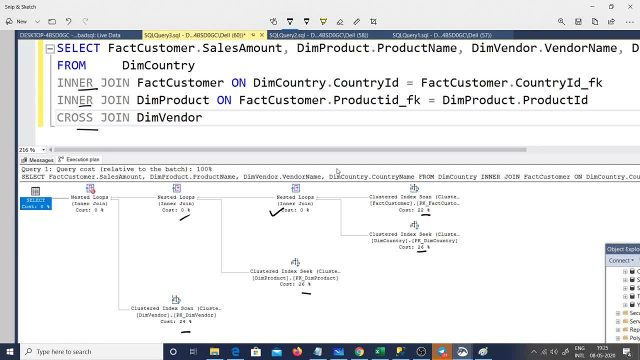 four percent and so on. This cost does not mean time. This cost does not mean CPU performance. it is a cost. This cost is calculated on lot of things. So you can think about: this is a matrix of SQL server, right? So this 20 percent means 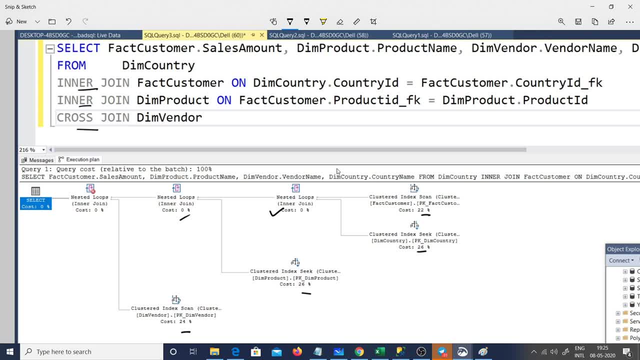 26 percent means the time is 26 percent more as compared to others. The CPU usage can be 26 percent more. operators and activities: Each one of these things, what you see out here are termed as operators means they are logic. For example, the first thing is: you can see, you have said: 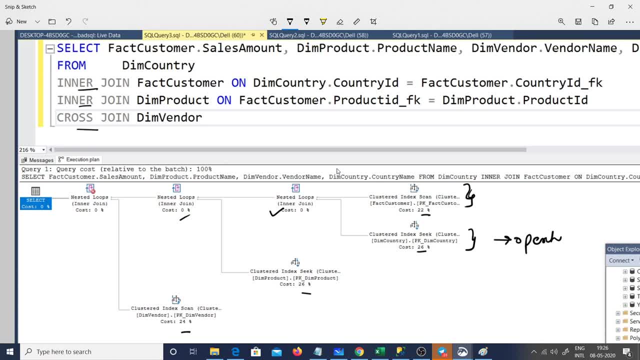 here you make a join on DimCountry, so that is the DimCountry out here. This DimCountry joined on FactCustomer, so that is the FactCustomer out here. and how did the join happen? It's an inner join, but he used the logic nested loops. look at this. There are two concepts. 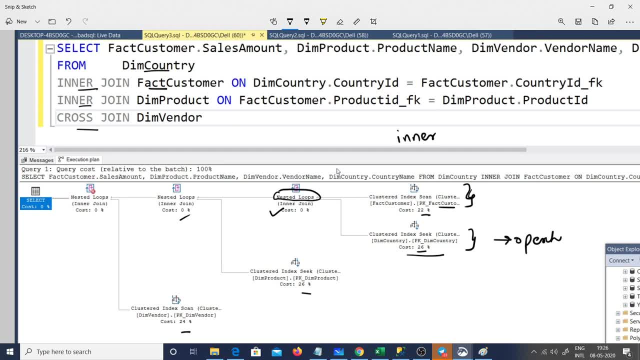 out here logical operators and physical operators. Logical operators means this is an inner join. so you want to go and write a logic. let us say sorting, Sorting is a logic. what you want to write, How you can write sorting logic. You can use bubble sort, you can use inserted. 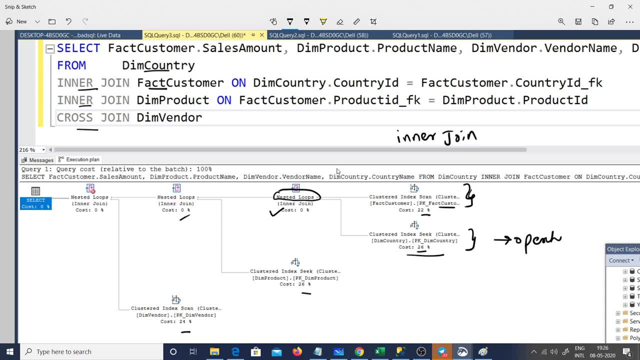 sort. you can use lots of sorts out there. Inner join is a logic nested loop, A logical operator, and to physically implement it he has used nested loops. What does nested loop means? internally Nested loop means he has a for loop and then again inside that. 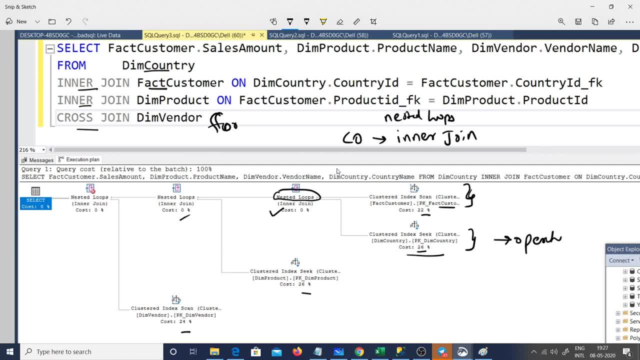 for loop. so he has a for loop. This for loop is probably on the FactCustomer and again there is a for loop nested for Here. he is saying that this is a nested for Now. this nested for can be very bad. Why? Because this FactCustomer is a transactional table On a transactional table. I don't want. 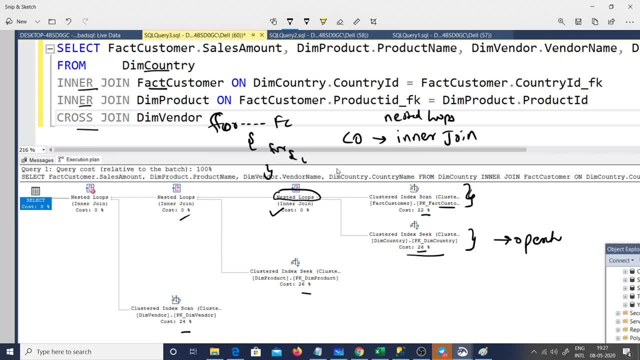 to see a nested loop out here. So you can see that this is something which I don't want to see, a nested loop, Probably. I want to see a merge join, probably a hash loop or hash join and so on. Again, you can see out here: we have the dim product. Again, there is a 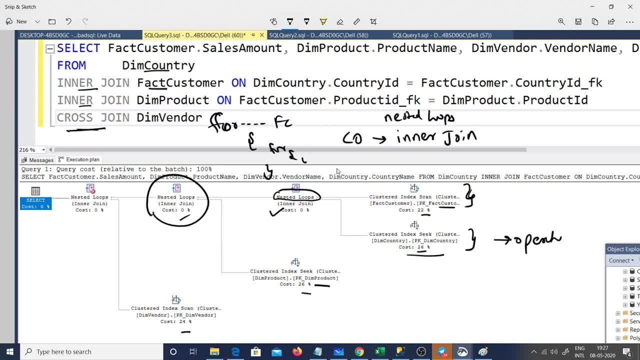 inner join and again now this one here is a cross join. So the you know your plan. Your SQL server was confused saying that damn it. like, what is this cross join? You know this? somewhere I clicked on those menus out there and gave out a cross join. So that red. 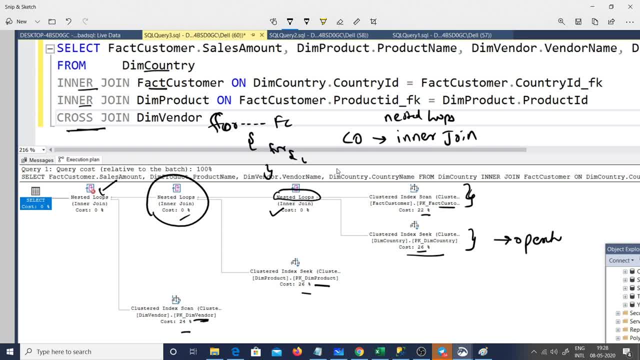 sign out here indicates that there is something terribly wrong here with the dim vendor right. So the first thing is, when you are reading this SQL plan, you have to read from the right to the left, Point number one: Your eyes should keep watching the cost out here: 22%, 10%. 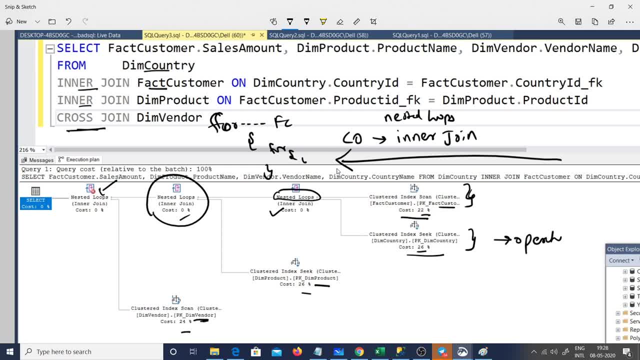 5%, 98%. Your eyes say, oh, why 98%? You should start thinking about it. You should start thinking logically. Your eyes should keep watching the logical operators and the physical operators out here, right? So that is one part that basically. you would like to go and see your SQL plan. 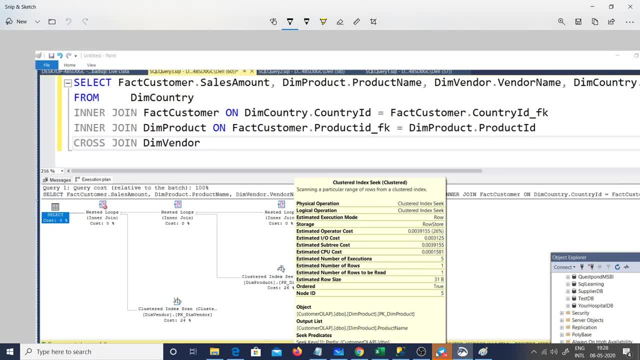 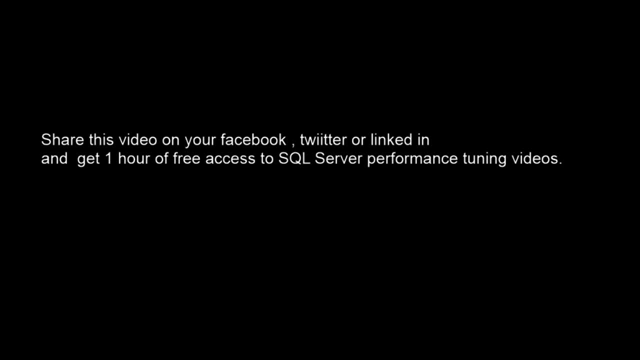 So any questions on SQL plan? If you have any questions on SQL plan, please go ahead and put down questions on the SQL plan And again, like so what we did first. First I went ahead and I said I want to hunt which are those bad SQL? I talked about using some profiler. 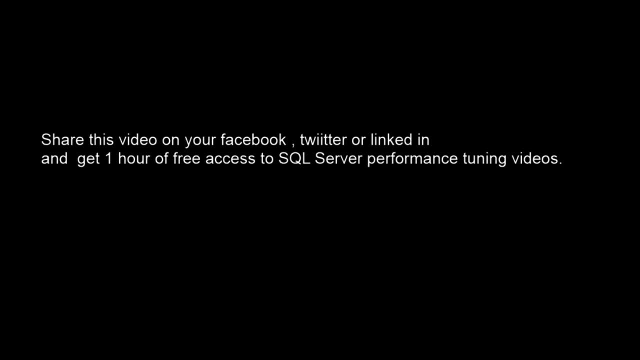 or you can use extended events, or you can use query store. Second step: once I know that this SQL is bad, I said, okay, like now, let me go ahead and understand. you know how the logic is right, Great guys. so any questions? and please, like you know, if possible, go through. 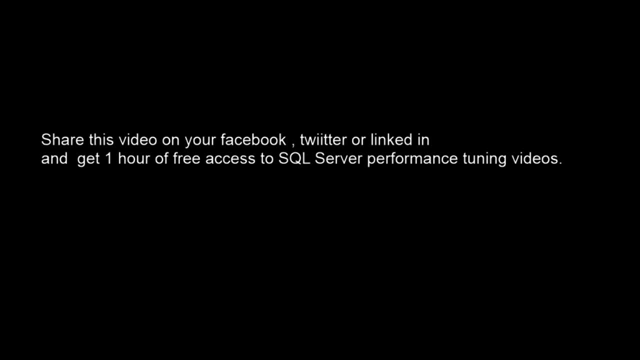 my SQL server performance videos. We are having the live training as well. Today also I have a live training on SQL plan. So on MVC and so on, we have the MSBI videos. do have a look at them. Any questions on till? whatever I have taken till now, I have taken two important topics: How to go and listen. 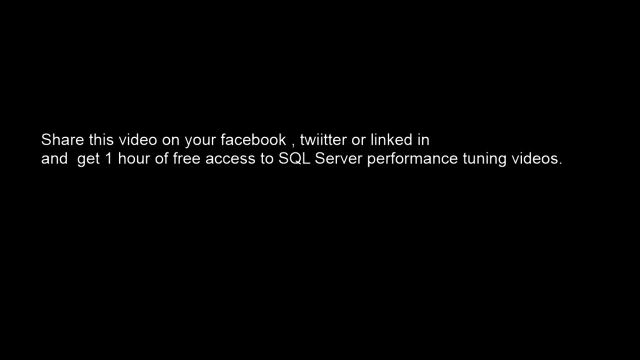 to the metrics of SQL and I will really look into that left side. Hey, Questpond support. can we next lecture? can we just test? you know why people are only hearing the left earphone? I am not really sure about this. I will check that part, So any questions out here? Yes, Yeah, so difference between 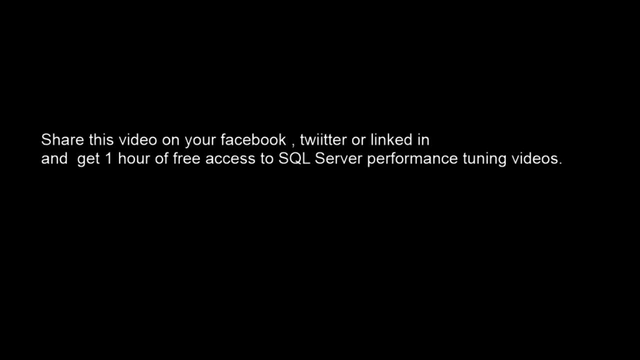 estimated and actual plan? I can see from one of the questions out here. See: estimated means it is not really firing on the actual database, It is just estimating it by looking at the current statistics. Whenever SQL server is running there is a current statistic which: 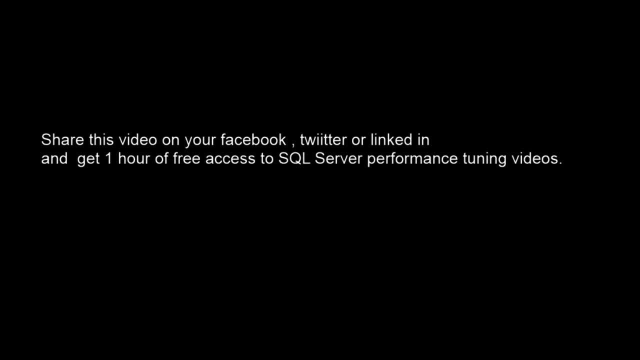 is created. This statistics can be stale. Actual means you will actually go and fire the SQL on production on means it will actually go and fire on production. It means you will actually go and fire on your database and you will try to get the metrics and always. 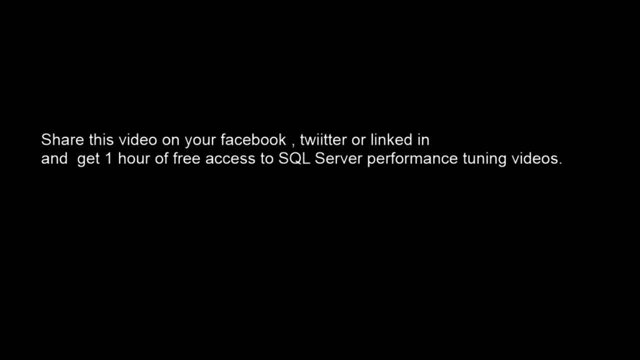 actual is not good. you know why? because if you are in production you do not want to fire that SQL. probably right, How to differentiate between physical and logical operators. So, physical operators, good question from Dakshesh here. Dakshesh, remember that physical operator? 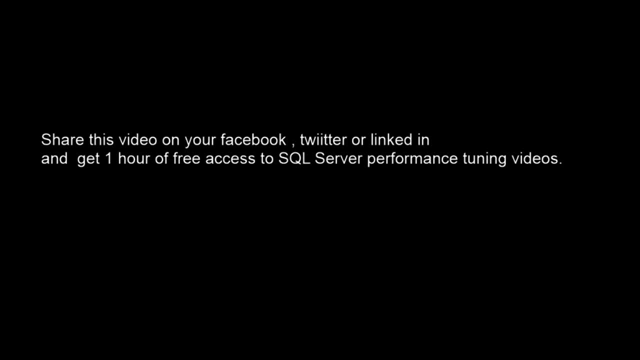 and logical operators are almost same, Almost they are same, like we were lucky to see the same. So whatever is down below written is the logical operator and whatever is at the side is the physical operator. So in my SQL query you know the in the bracket in the bracket. 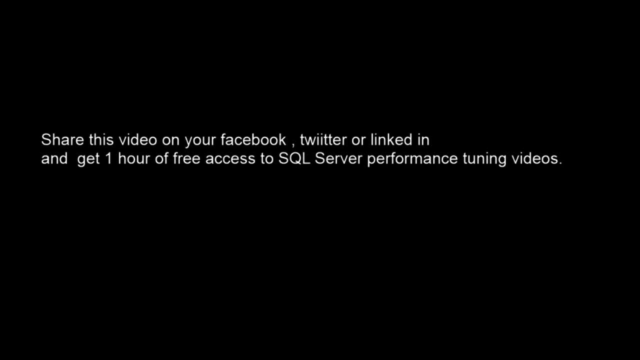 you know, whatever was written is the logical operator and on the top of the bracket, whatever was shown is the physical operator. If the cost is high, does it means we have to look into that? No Vidya like. So first thing, guys, you know this is very essential. 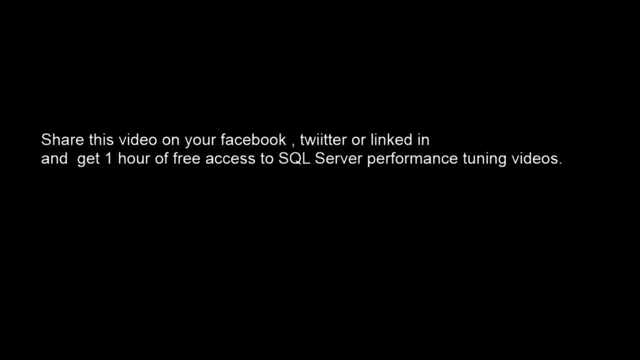 one is: you know, I have, just you know, this is like 3% and 4% of SQL performance tuning. really, It is just to get started. you warmed up right, So good question, Vidya. So if cost is high, should my eyes go out there? No, like, see, remember, performance tuning is an art. 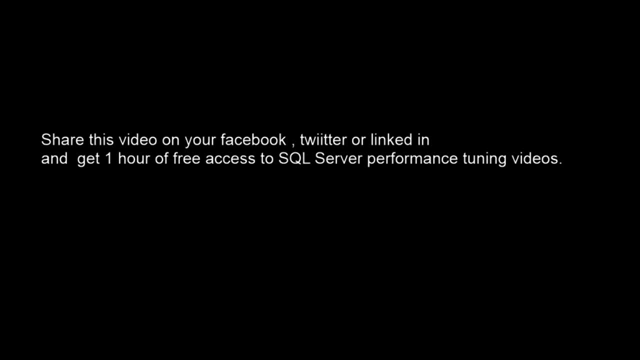 It is a kind of a sixth sense, It is a kind of an experience. So at the first time you won't like. you will find that all the SQLs are bad. Sometimes you go and you keep looking at plans. you go on circles and circles and you don't really find out what the problem. 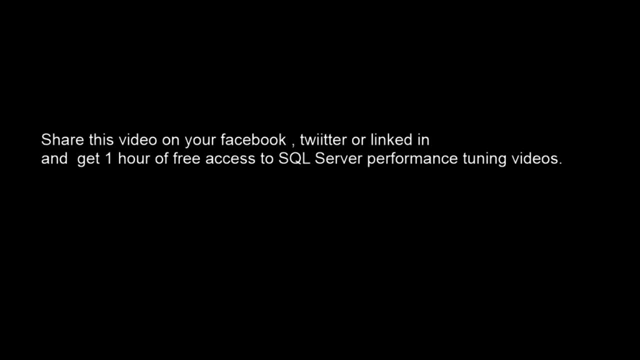 is So it's really an art right. The fact is, logical operators and physical operators are one of the factors right. In the same way, I will show some other factors also. So it is lot of things. for example, when a doctor looks at a patient right, he says okay, like, so what is it like? his heartbeat. 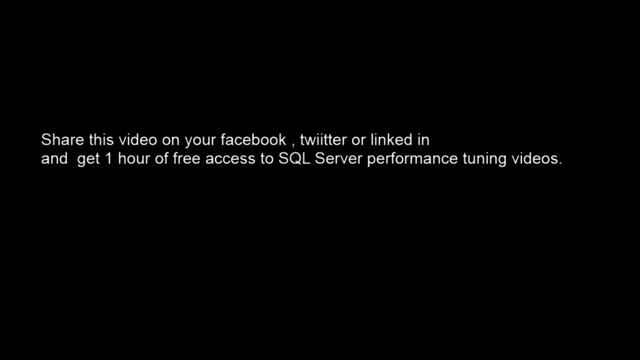 this, this, this. There is some kind of a human intelligence as well on the top of it. you know the metric that you need to put out right. So that is definitely one of the operators, but that is not only the one operator which I will see. Yeah, so good. So, Joseph, that's. 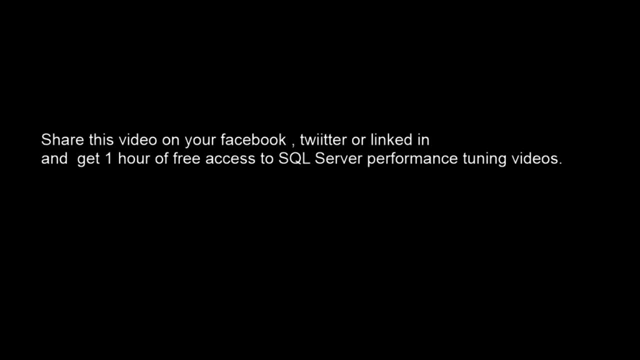 a good thing. So, on this, if you are a beginner of SQL, this is really a higher end or higher end training Joseph. So what you can do is, Joseph, if you want to get started with SQL Server, if you go, if you can Questpond support, can you please pass on to Joseph, sir, you know the the link. 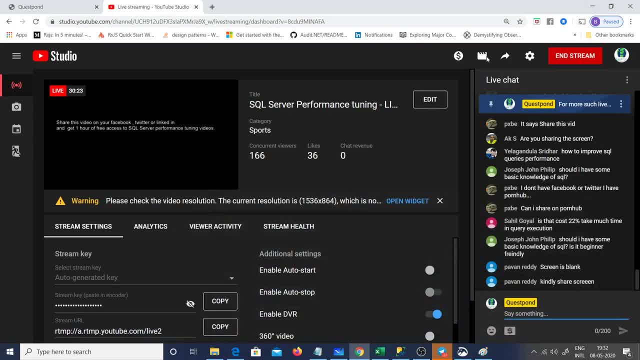 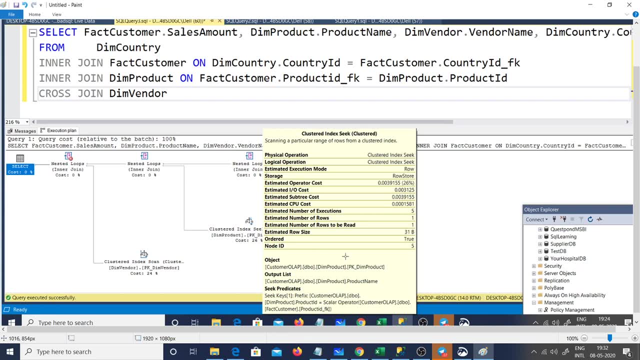 of our freshers SQL Server. So people are new to SQL Server. you can go and you can watch the basic SQL Server training videos out there. Okay, guys, now that is one part. that was one part. you know, watching those operators, watching those things, right, There is a other thing also, which your eyes can really flow out here. 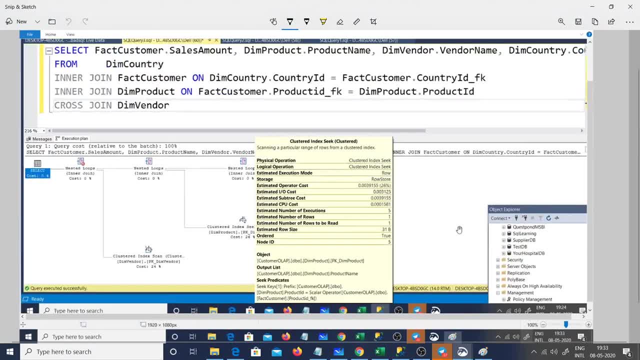 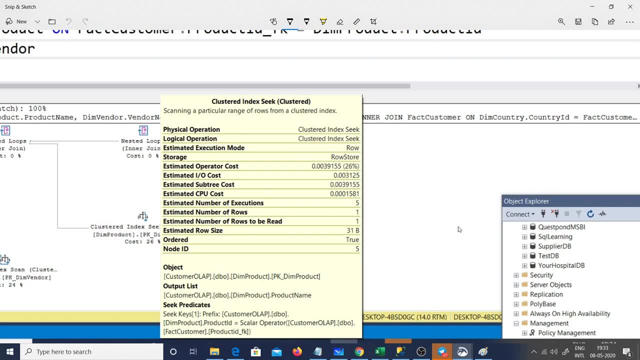 okay, let me go and zoom. you can see here I have zoomed in. So when you go and move out your mouse out here, when you go and go into any one of these operators, you will see more details of it, right? So, for example, you can see out here we can have a just a basic understanding. 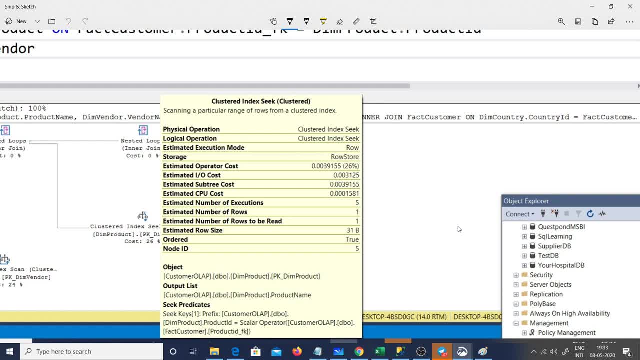 of it. The first thing that you have to do is you have to go and move your mouse out here. When you go and go into any one of these operators, you will see more details of it, right? So, for example, the first thing is you will see out: here is there is a physical operation and 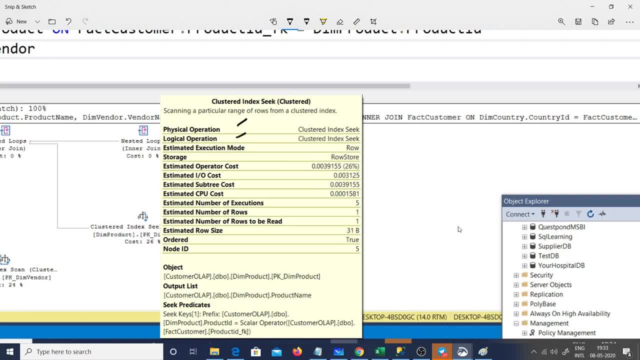 a logical operation. So I have already said physical operator and logical operator. somebody was also asking me how to know what is a physical operator. whatever is inside this bracket, or also if you can go and move your mouse on this here, it directly says: you know logical. 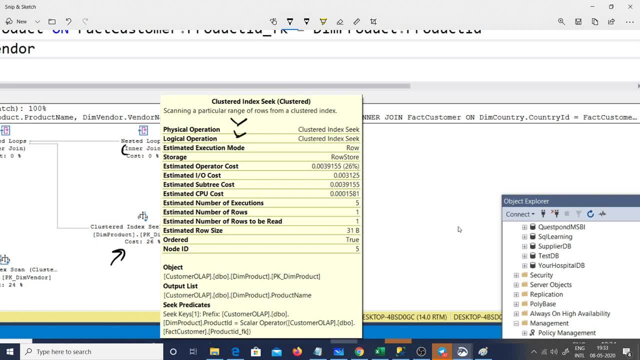 operation and physical operation. So this is one part: Estimated execution mode. this is one more like good thing to look into. one is: you know, row by row estimation. So, like you know it, row by row has been executed right. So. but another one is: you know, sometimes you would like to go and see a batch here. Sometimes. 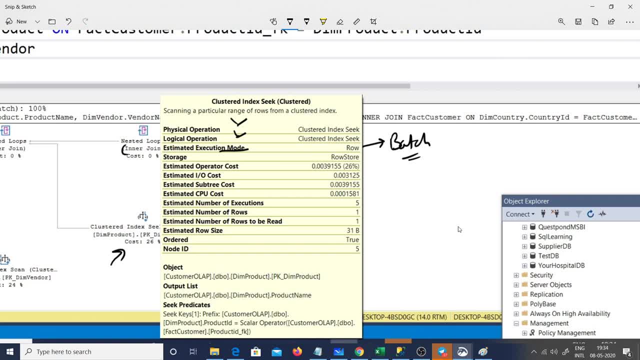 you want to see that. no, like I don't want to do row by row, I want to do a batch, probably right. So again, there are two things which you can look out here: row and a batch. We will not discuss. you know, when do you see a batch here? that is for later discussion. 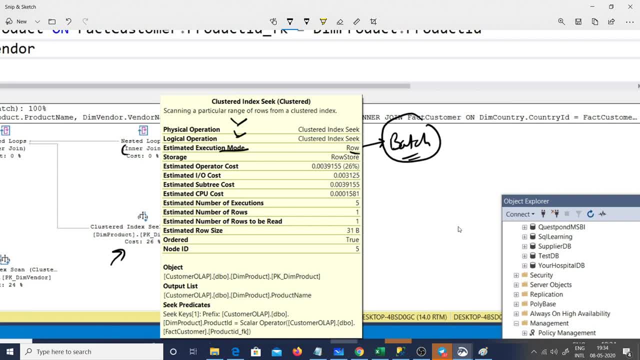 right, Leave the storage for now. Operator cost. I think this we can see on the screen out there. The next one is IO cost. IO means how much read and write he is doing on the hard disk. So this SQL, So this SQL. 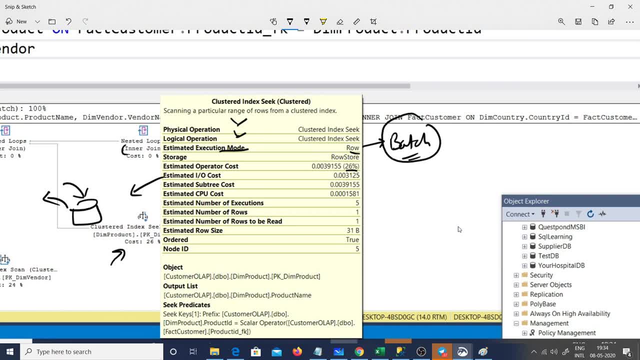 Is definitely a simple select. So you can see the value is 0.00312.. So it is actually doing just a read. But let us say, if you had a SQL which was also doing an insert update, then this input output would be very high cost, right? You can see CPU cost. So like: 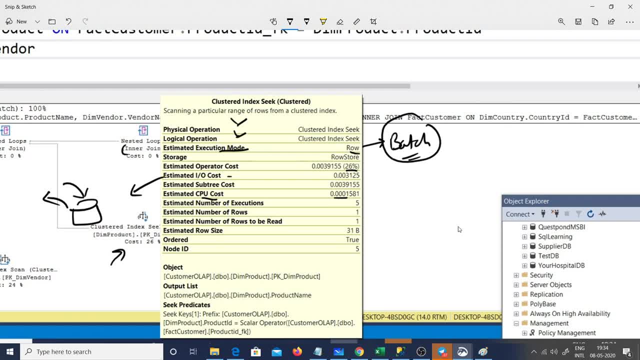 how much processing it has taken. So if you see out here, this is like at the end of the day, what do you have like? it is going to go and use your computer, right. So in a computer it is going to use CPU, It is going to use your hard disk, right. 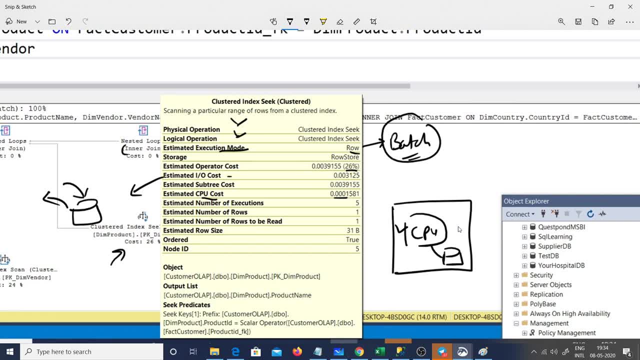 So this CPU cost? you know what you see out here is nothing but this one. And this input output is nothing but you know when it starts writing to the hard disk right. So both of these cost actually talk about the physical devices you know how they are utilized of. 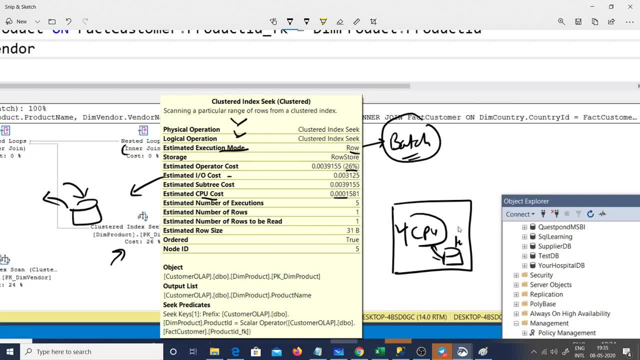 your computer Right, so estimate number of rows. So like at this moment, probably it is having one row, but it if you see lot of rows out here, like like this, that means something is bad, Something has not been filtered right. So let me go out there, Let me see if I can show you some. 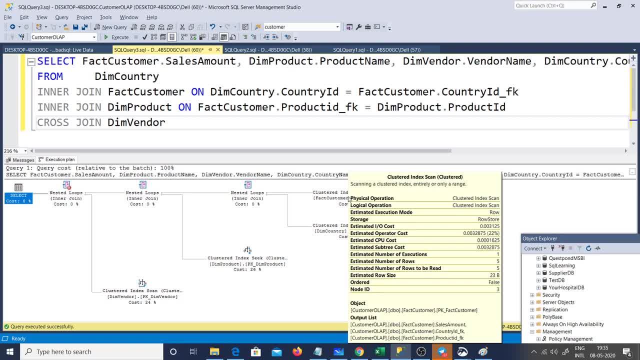 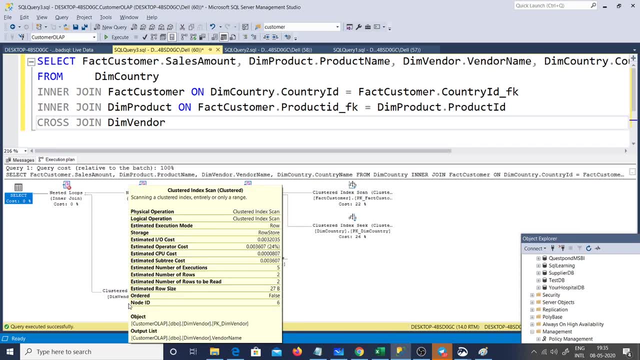 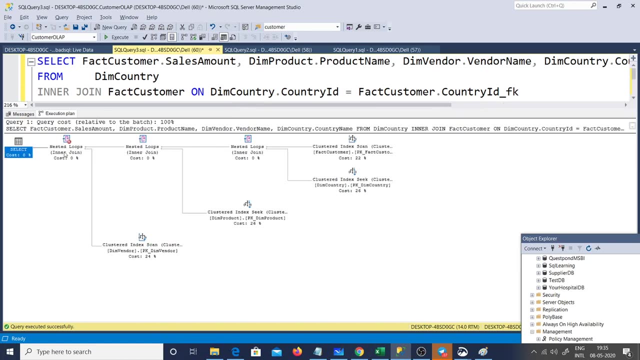 more exciting things. Let me see. you can see, here I am moving my mouse. Look at this. This is a bad one. This is really a bad one. You can see there is a red sign out here. How about going and dissecting that? So let me go and put a print screen out there and let 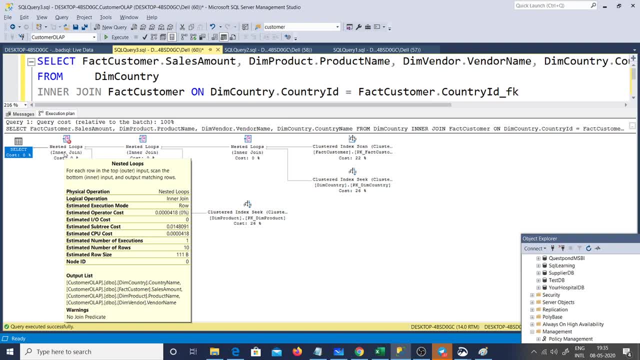 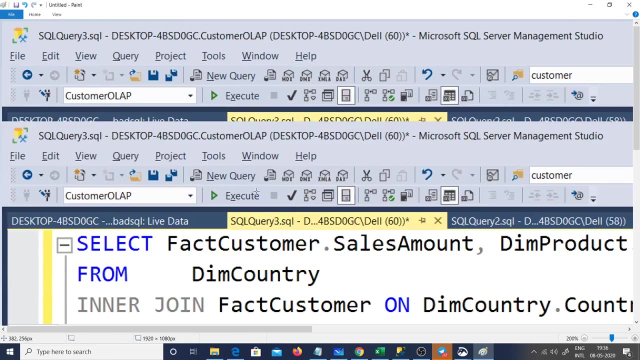 me see if we can really dissect that. Okay, You can see there is a print screen out there. You can see it is showing a red sign out here For each row. it is a nested loop, right. Look at that, you know. let me just control print screen function. print screen. I am so sorry. 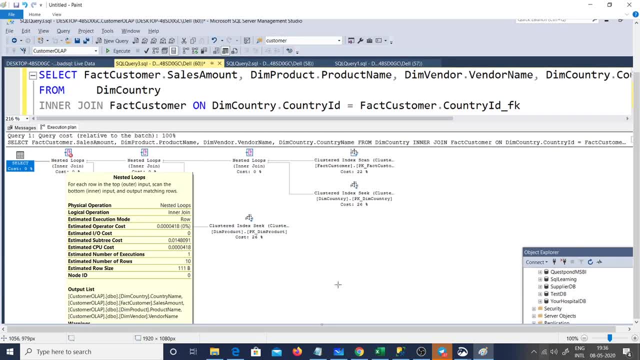 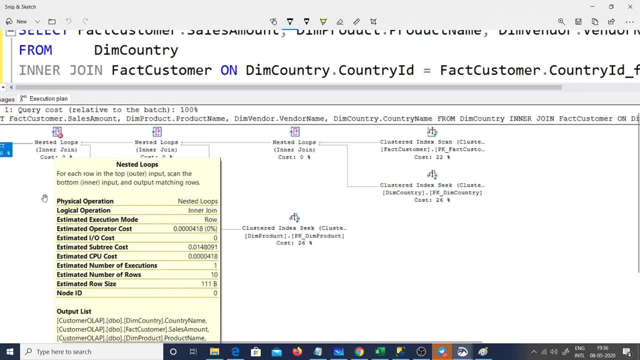 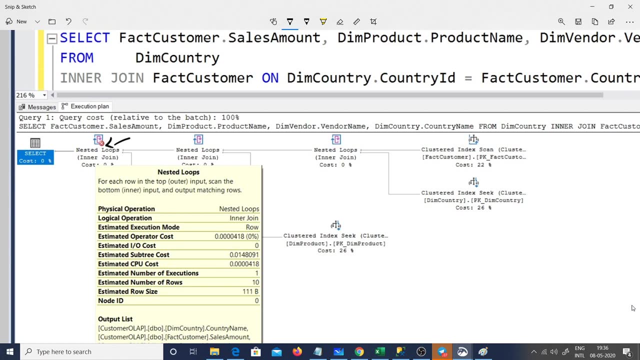 guys, you know I have just taken up some SQL which was lying on my database. Must be, I should have come more prepared, But that is fine. Okay, here it is. I am particularly taking this. It is showing properties more. Why? because I see a red sign out here, So we can see something. 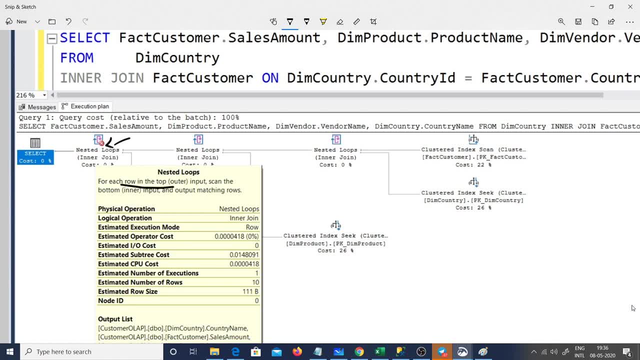 nested loop For each row in the top outer input output matching it will show So that you can see nested loop out here. You can see number of rows. It is showing ten rows out here. So definitely I do not have too much data out here, but if it is showing large, 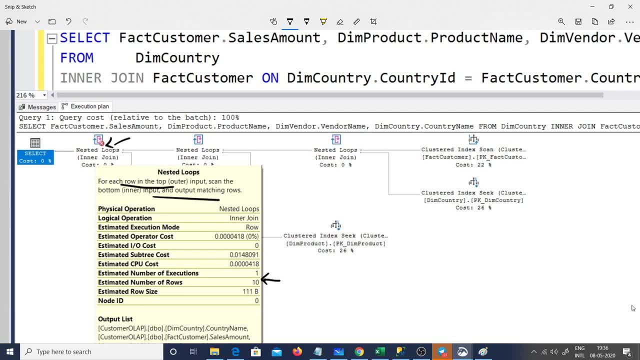 number of rows must be. you should put a filter somewhere, right, because taking so much rows and doing a scan, it does not make sense. So but here it is. It is not showing me out here. Sometimes I think what I let me. let me go out there and I executed. I think I executed. 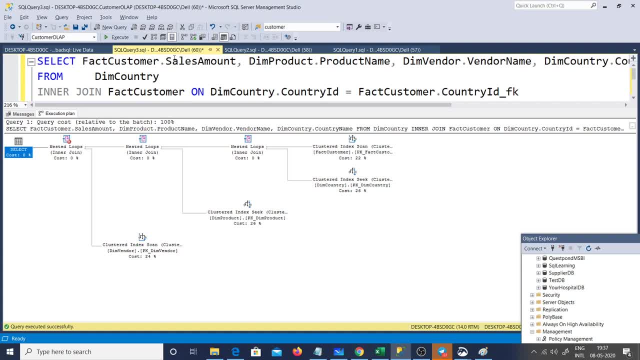 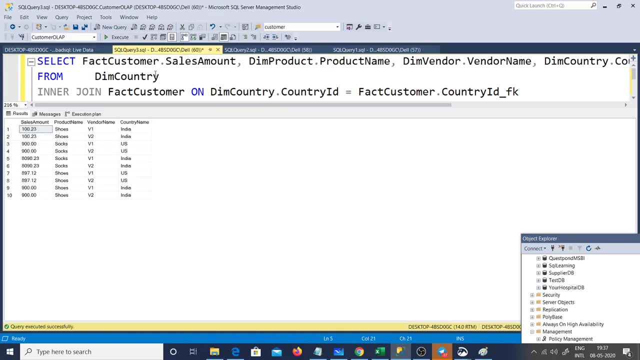 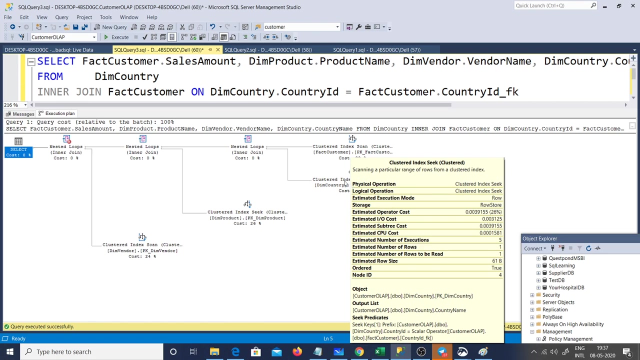 let me do that. I executed an estimated one. how about? okay, let me do an estimated one. Let me do an estimated one. I want to see my estimated plan. What happened? estimated? can 갈 estimated, estimated? is that estimated, estimated, estimated? oh well, it's not showing anything out here, must? 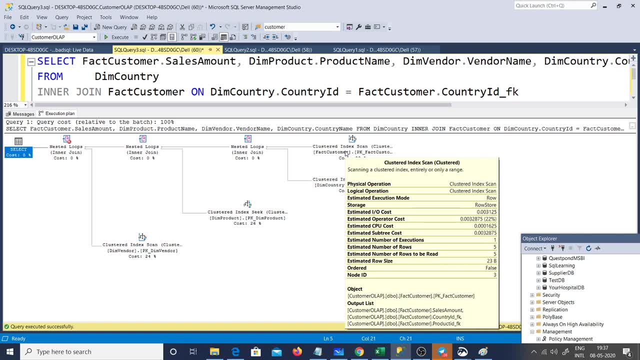 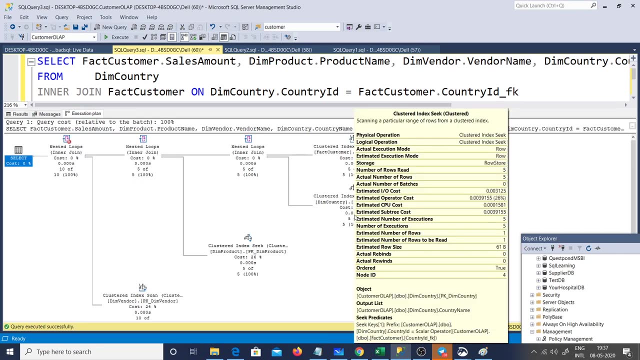 be. I need to be, yes, estimated. let me see over here actual two minutes, guys. I want to show you one of the metrics which are really, really used wherever I go. yeah, that's what I wanted to show. let me do a print screen out here and let me show. 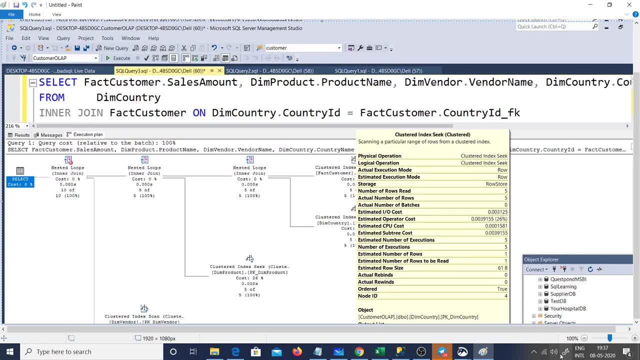 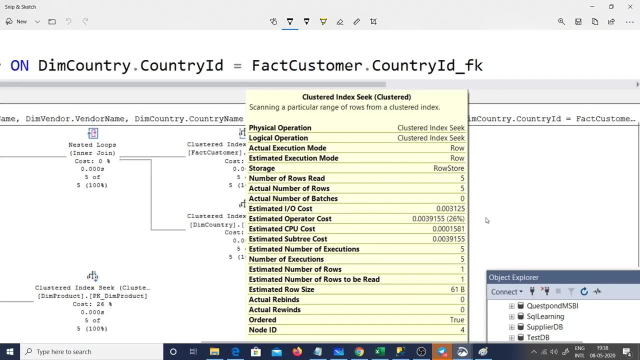 this okay, right, if you see this plan out here, you can see some more details. this is the actual one, right? so, in actual one, what it is saying, which is one of my my eyes always catches out here. it says that number of Reds, number of rows, read: 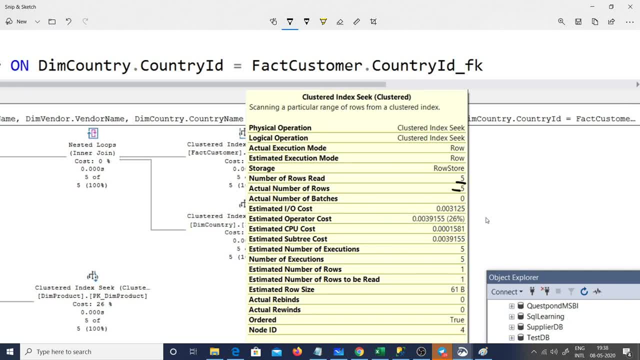 are five. right, actual rows read are five, but you know what? he thinks that the estimated rows should be one. you can see here there is a mismatch: the number of rows which are actually there, number of rows which are actually read, are five and the estimated one he thinks is one. so that means that my statistics is out of date, remember. 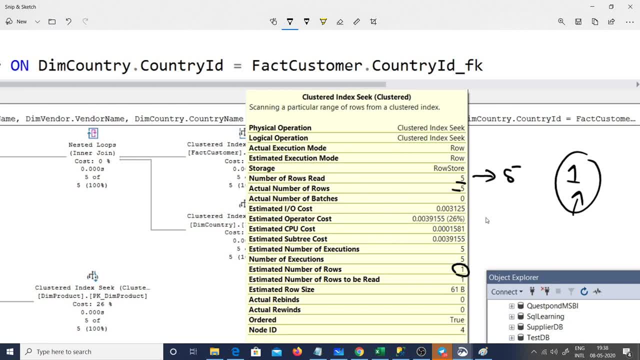 the SQL Server has statistic. this is one of one of the things which I really catch in my eyes that the SQL Server thinks, depending on this statistics, he thinks that only one row he will get, but actually five rows are read. so whenever you see a very huge 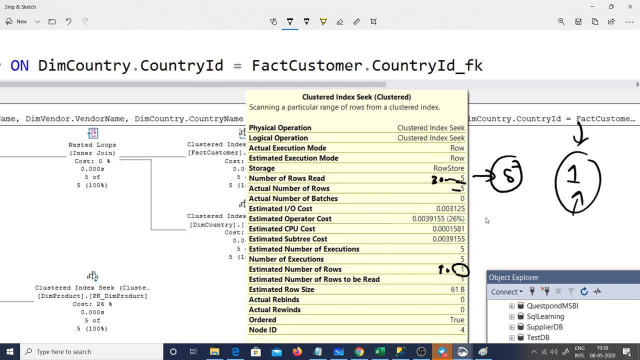 number out here, like thirty thousand something, something, and you see only like hundred rows. something is bad. right, then you should go and you should try to upgrade your, update your statistics, right? so these are two, three things I will see. the first one is: I will see the physical operation, the logical operation. 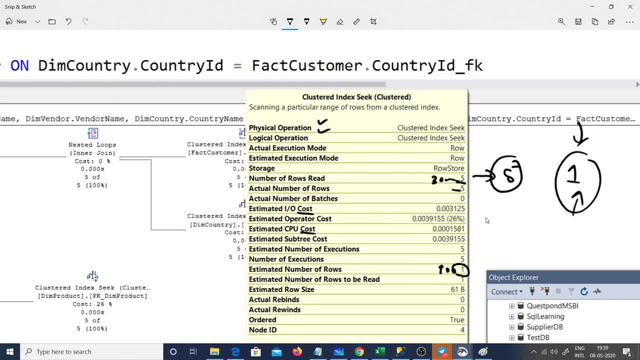 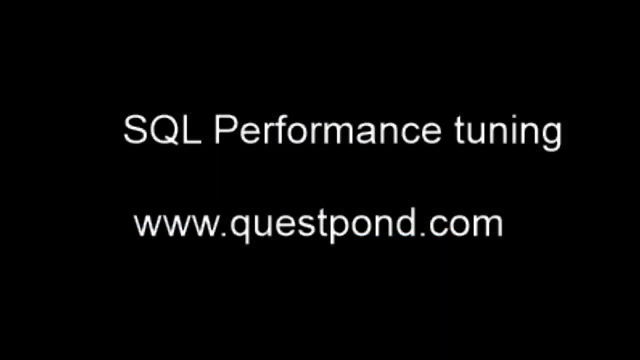 I will see the CPU cost, I will see the input output cost and I will see that. do I have a plan mismatch? do I have the statistics mismatch right? so as any questions out there, any questions on the deep properties which I discussed here. so there is a question here from Kishore. so the inner join causes. 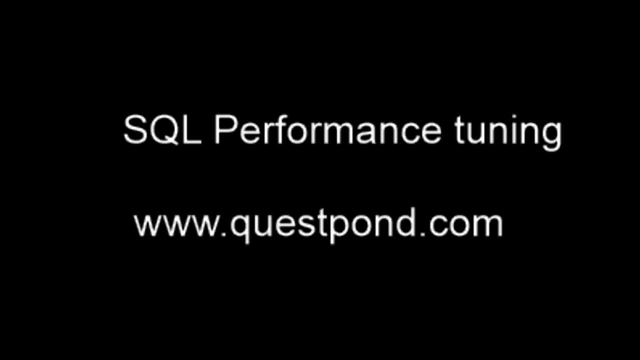 nested loops. yes, see, inner join can cause a nested loop, it can cause a hash join. it can also have something else. you know there are three, four different types of things out there, so it can have different ways of executing it. today we will not discuss that part. is nested loop good or is hash join good or is merge? 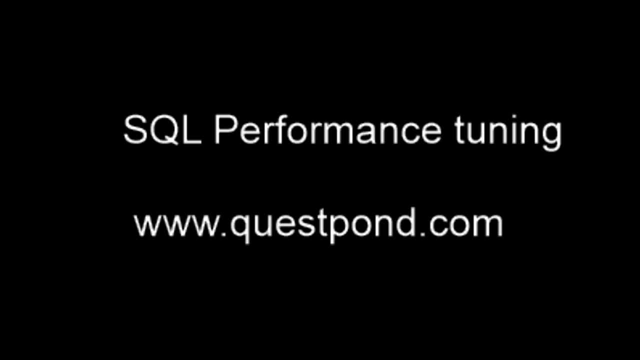 join. good, that's a discussion for some different thing altogether. actual and estimated, was it five? no, hang on. let me look at my eyes. okay, estimated number of rows are read are one and actual number of rows are five. so actual rows are five and means what that? actual number of sit, the number of rows read. the number of rows read is. 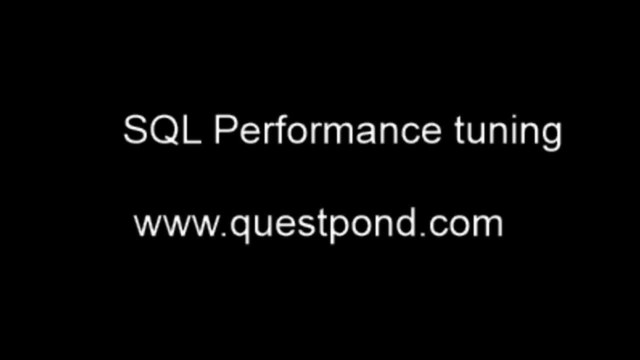 five, right, and the actual rows are one, you know. so if there is a mismatch, right, ooo Penel, oh my god, Penel is here. oh, Penel, the way is here. okay, sorry, Penel reading was it's actually reading five rows and actually are both five. okay, sorry, oh its, if Penel. 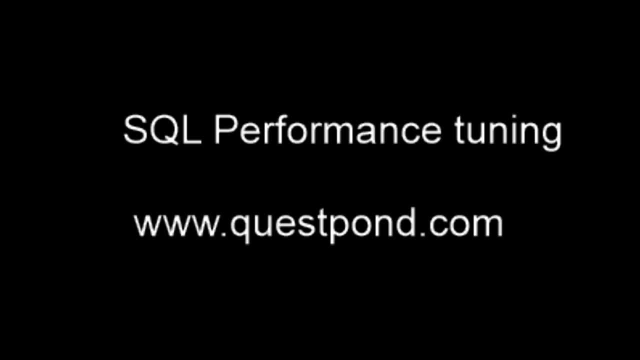 is saying: I'm sorry, Penel, I must have read it. you can also, instead of Sorry, hyung, think I must have read it. I must have beautifully read it, Penel, just like anyone else. I am sorry, alcoholizzed, regretting. Oh, Penel, you want to imagine an interview to talk about? you. Oh, Penel, you want to imagine an interview? okay, try this. everyone would becken awkward. cannot see my ass, cannot seeembermana, like some wif에도grippi wifedom c? h, 아니면 mind that Penel does not know if we went to India. you know, flew inspiration from many others. 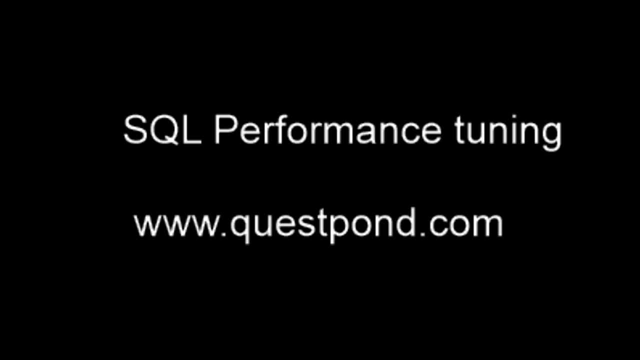 So Pinal Davey is here. I am so honored, Pinal Davey. everybody knows he is one of the forefront when you talk about SQL Server. Thank you, sir. Thank you with all respect. you have come today on my session. Definitely I am a jack of all and you are like master of SQL Server. Thank you very much to come on my session. 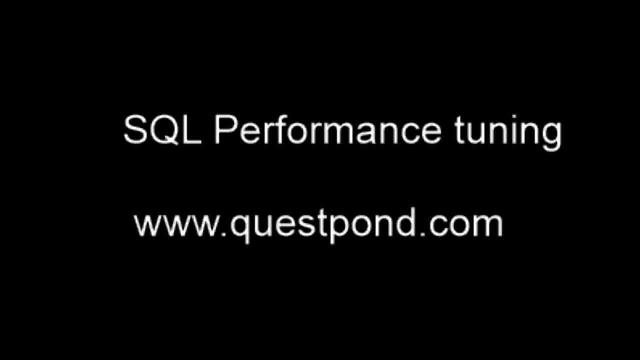 I can't see the SQL query duration and SQL query log. So, Gopal sir, if you see, in my previous part of the video I have shown that- how to go and see the duration. So when you actually go and run an extended event or when you go and run a profiler, you know that duration actually gets captured. 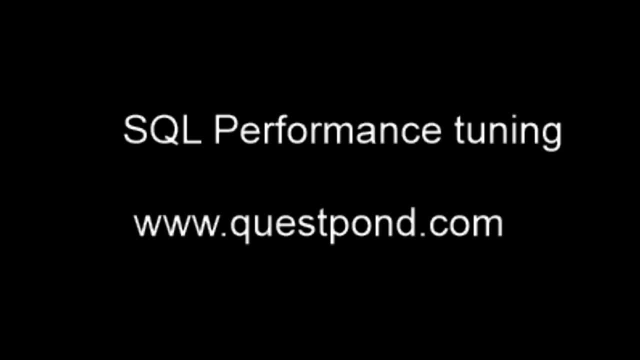 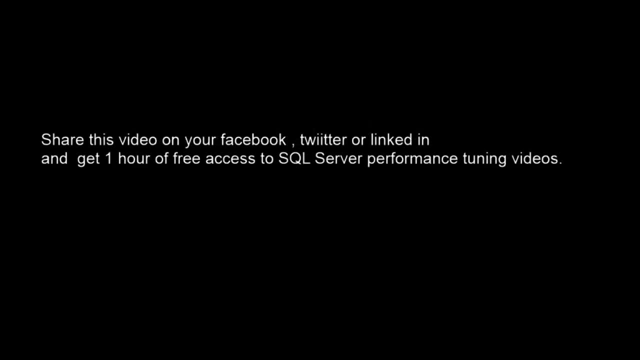 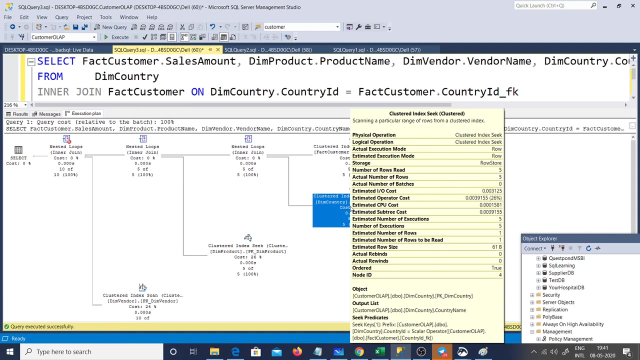 Yeah, and the number of execution is five and actual reading: Okay, actually, Pinal, let me just show out here. So I think, yes, I must have mistaken out there. I am sorry, But the point is, Pinal, sir, what I was making out a point out here is: let me go and show out here. So there, it is Okay. 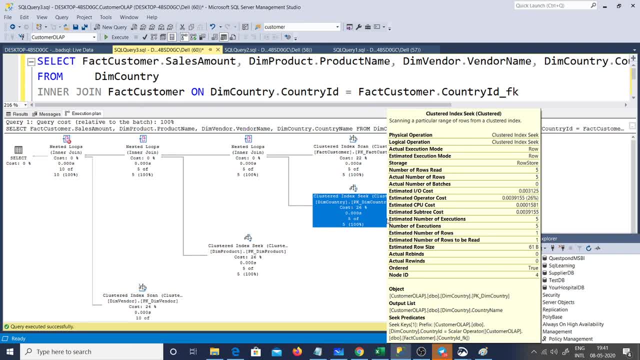 Estimated number of rows. that number of rows read, actual number of the number of rows read is five at the top, and the estimated number of rows to be read is one. So that's what made me, Pinal sir, think you know that. 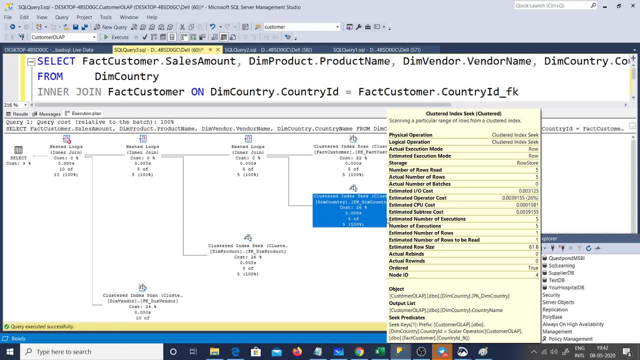 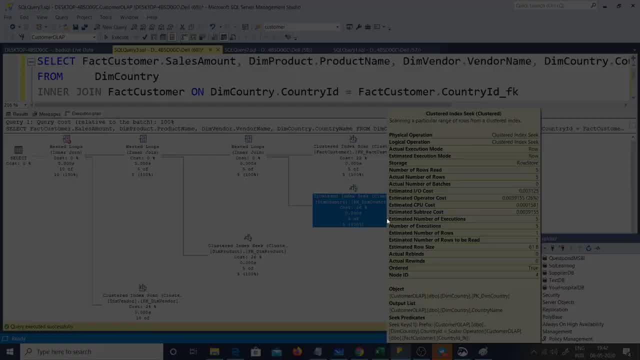 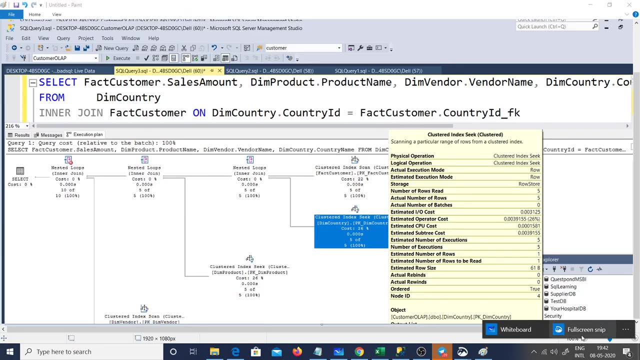 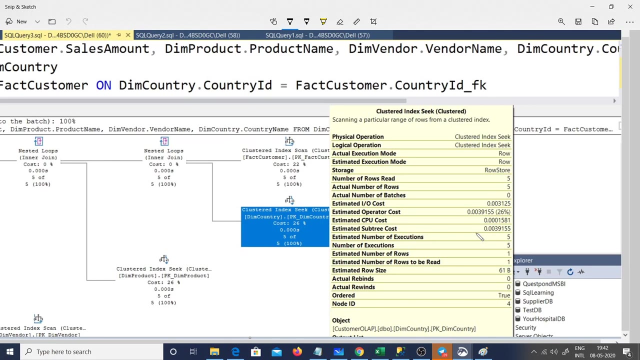 it's not the execution, is not here The number of execution. I am not seeing Number of execution. I understand, So let me print screen So I can be wrong. and so here actually, just you know, with all respect, you know that Pinal sir has talked, so I need to. So this is the number of. 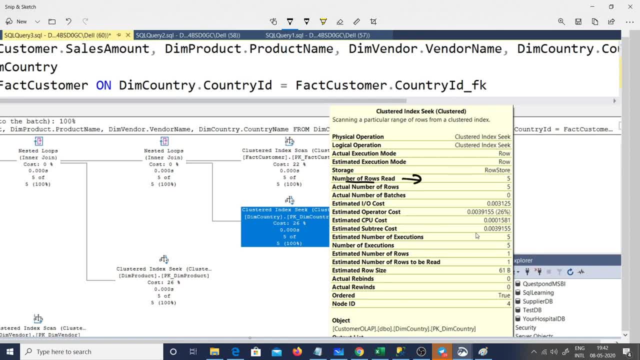 rows read. this is 5 out here, which I see, and if you see out here the estimated number of rows to be read he is thinking is 1, so must be. that made me think that the statistics are out of sync. The number of execution is different. definitely, this number of execution. 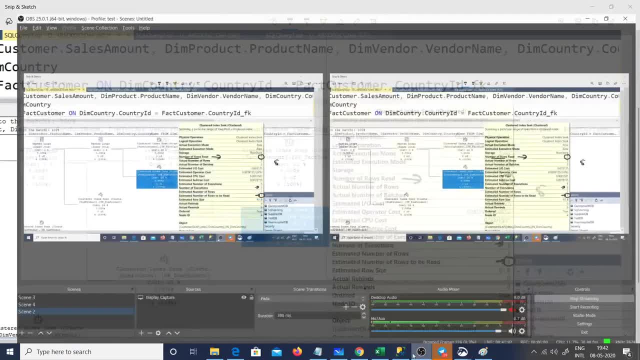 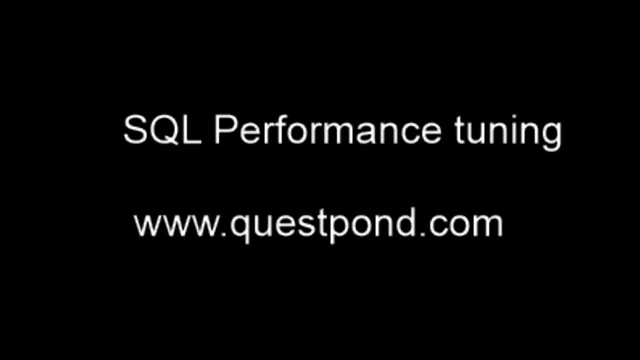 that is a different part. execution means it is something different. See some other questions out there: 5 into the 1 row, 5 total: yes, yes, yes, then I got it. yes, Penel sir is right. yes, yes, yes, Penel sir is right on that matrix. thank you. 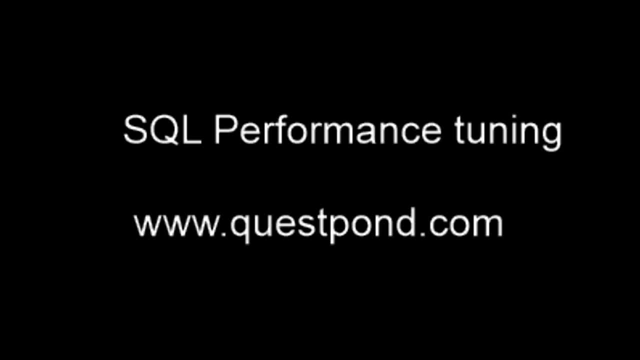 very much. yes, but that is again Penel, one of the things which I watch. sometimes they really go out of sync. that is what I was trying to say. Thank you very much, guys. so I think we are almost. this was a 30 minute session. thank you very much. 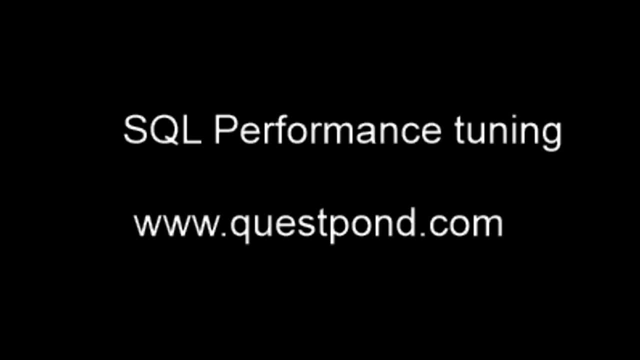 40 minutes of session. so any questions out here, any queries. let me know if you have any questions. So there is one question out here: should I use a profiler or should I use extended events? I would say that please go ahead with extended events because they 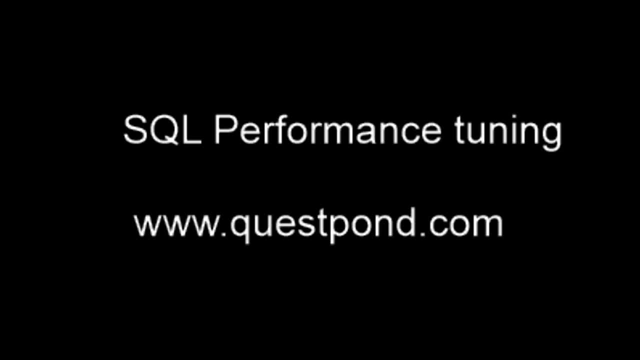 are more light weight, Right. so thank you very much, guys. thanks a lot, and please do go ahead and visit my site here, questpondcom. and we keep doing trainings every evening out there, sometimes on MVC, sometimes on angular, sometimes on react performance tuning. 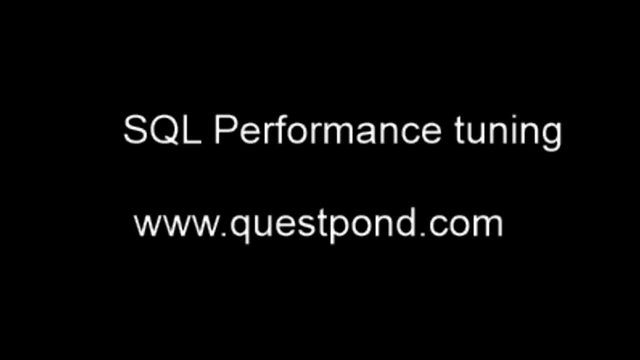 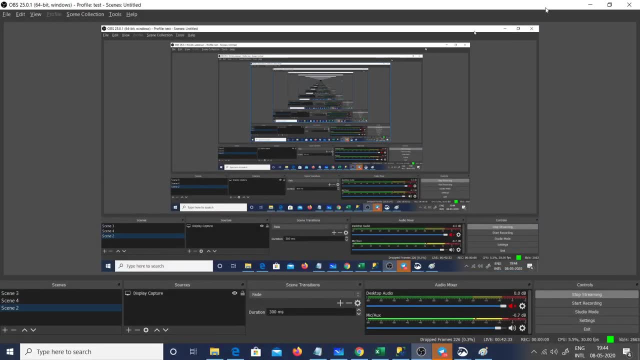 data structures. so there are lots of things going on out there. you can go and you can visit my site. you can go and, in case, if you are already a questpond member, I would really suggest to go through each one of these videos out here, whatever possible, remember everybody. 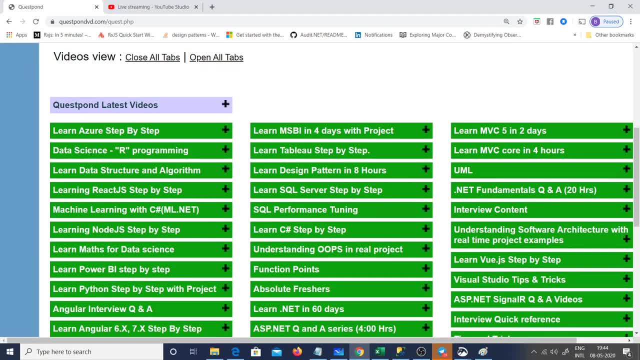 this is the time you can upgrade yourself right, so you can see so many things out here: learning Azure, learning MSB. specifically, if you are an SQL server guy, I would really suggest two things. one is go more in depth into SQL server today also. I also don't know. 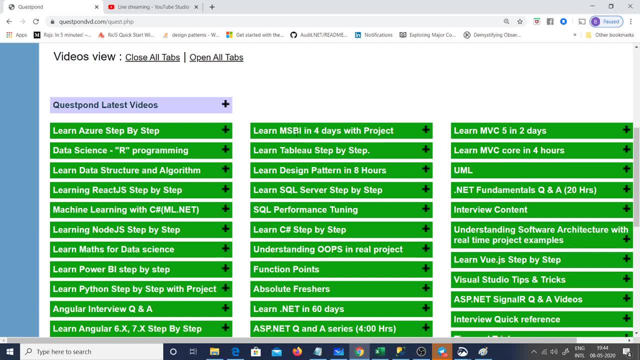 SQL server, as Pinal sir said, right into execution plan. into execution, right? my eyes just went out from there, right? but the point is, SQL server is a sea out there. even if you spend your whole life, you would still not master it, right? so I would suggest MSBI again, people. 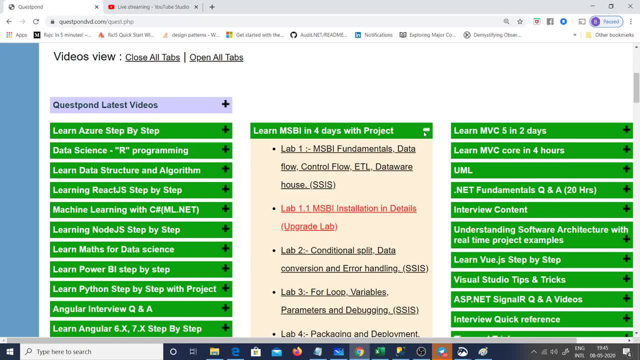 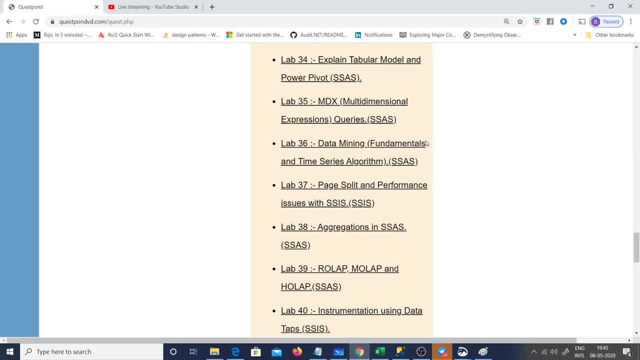 who are into purely SQL server nowadays. business intelligence should be part of it, right? so MSBI, Power BI. so you can see out, here we have this use tutorial series which is like a 40-50 videos which are dedicated only to MSBI. so I would really suggest just see one. 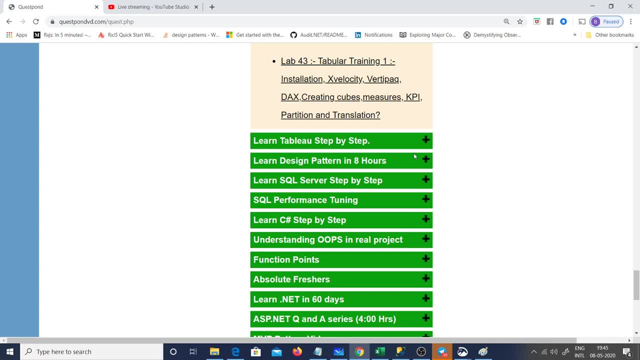 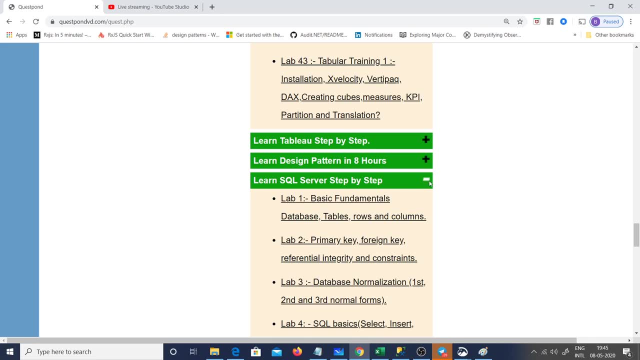 video in a week. I don't want you to see like 40 videos. it is impossible: one video, two videos, as far as possible. right second is SQL server. we have a complete, basic, fundamental SQL server. then we have SQL performance tuning and the next thing which I really want to. 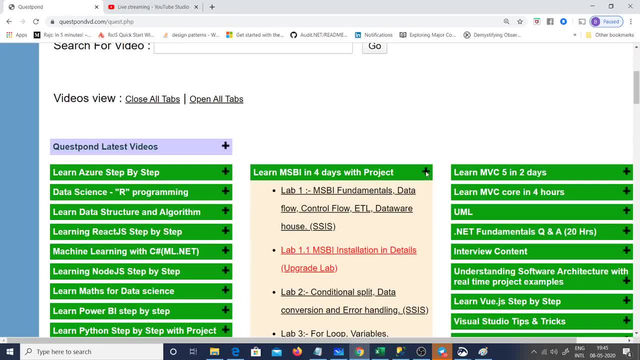 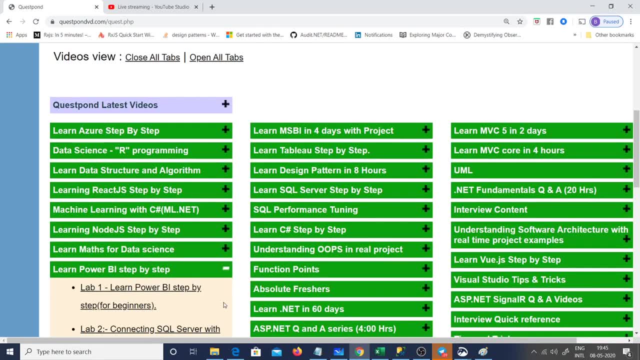 suggest for SQL server people is Power BI nowadays. Power BI, the visualization tool, Power BI. so again we have this Power BI out here. right and yes, why not extend yourself for data science? so in SQL server, you can see there is R and Python support nowadays. 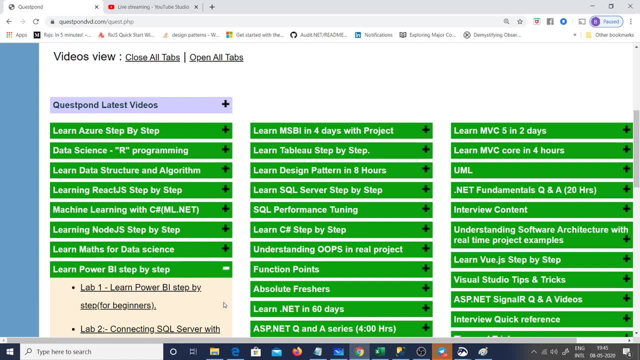 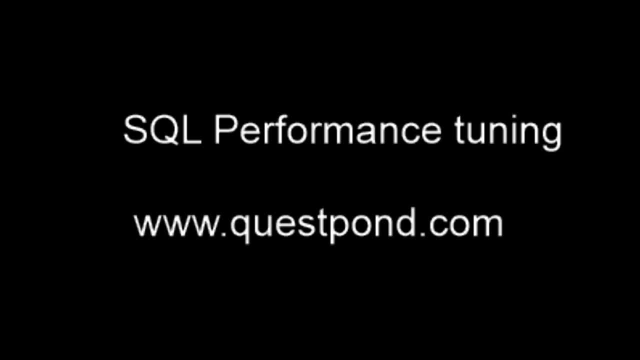 so lot of people are executing those models etc over there, right. So thank you very much, guys, thanks a lot and thank you to come to this session out here discussing. I can see that we have like almost 200 people out here. thank you very. 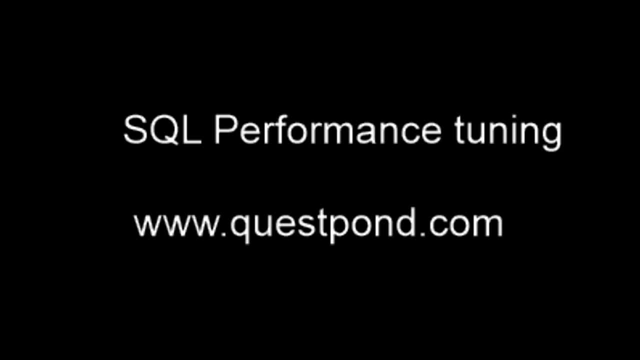 much Pinal. it's coming from you, I am so glad. but what Pinal sir said is absolutely right. it is number of execution into the rows. that's how it should be. but the point, what I am saying out, is that sometimes you know that actual and the estimated they go completely. 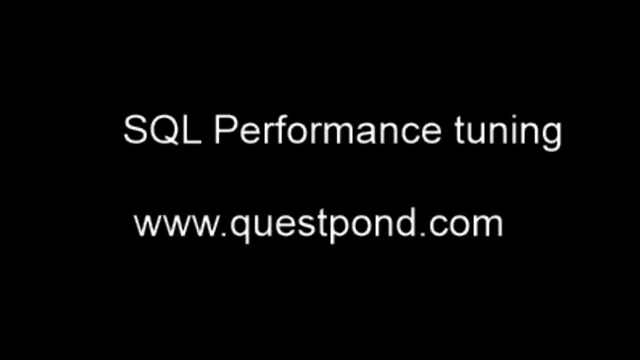 out of sync, then that's the time I see that must be. the statistics are not up to date, right? I need to go and update it, Okay, Okay. So could you name some physical operators and logical operators? I will take the last. 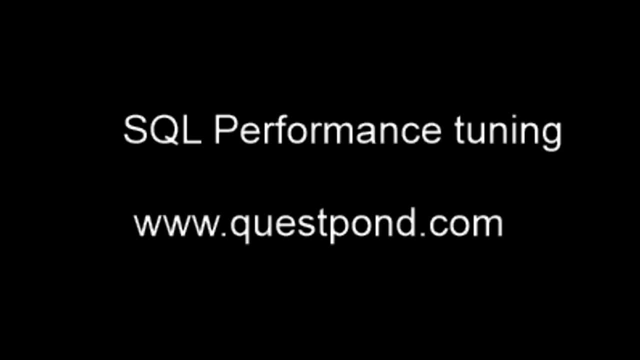 question out here. you can Google, you know you can Google out there logical and physical operators and there are holds of. I remember there was one MSDN link out here which had the huge references of the logical and physical operators. I can just pull it out for you. 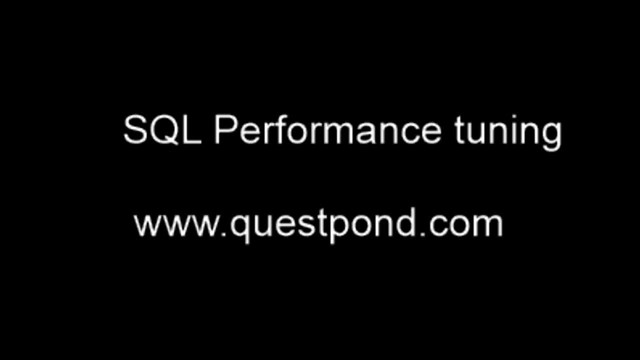 okay, there it is, So I am pasting that link. Okay, So I am pasting that link on the chat. you can have a look at it. So, but I would suggest, you know, do not try to look into those logical and physical operators. 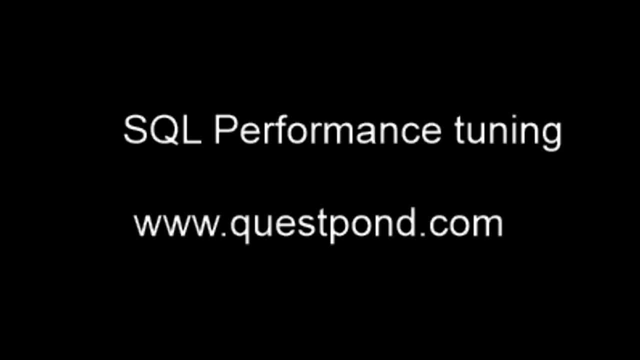 take ten of your favourites. take like five or ten, you know, let experience build on it. Okay, Gopal sir, I will take your question. what did? I did not answer your question. Gopal sir's question. let me see at the top. please help to answer Gopal sir's question. I will. 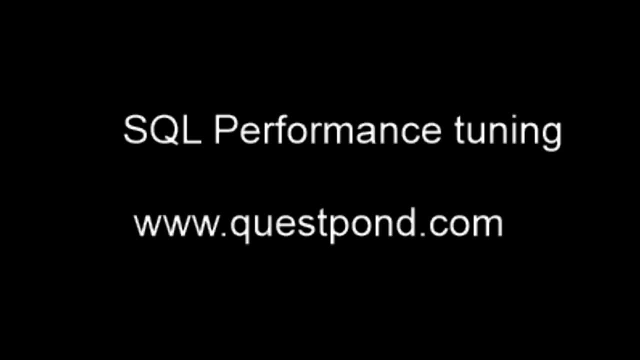 answer Gopal sir's question and then I will close it. there are so many questions out here. Okay, Gopal sir, I must hi in session events. I cannot see SQL query execution duration and SQL lock. SQL query execution duration is seen out there. I actually showed it. I.